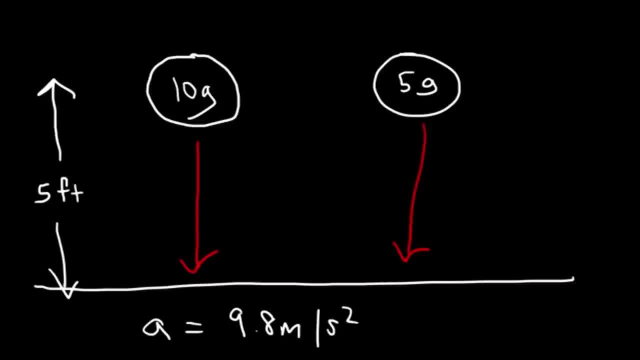 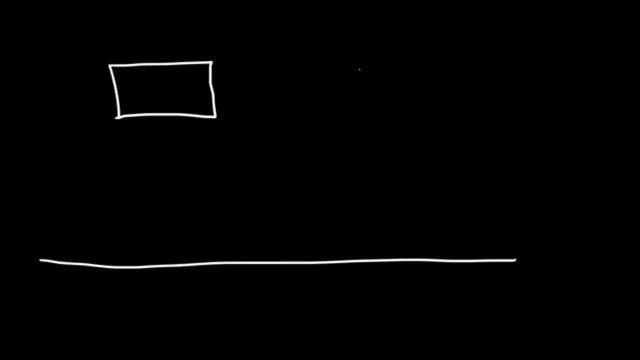 But because everything is the same, the height is the same, the acceleration is the same. if you take away air resistance, both objects will hit the ground. Now let's say if we use an actual demonstration of a brick versus a flat piece of paper. So the brick is a lot. 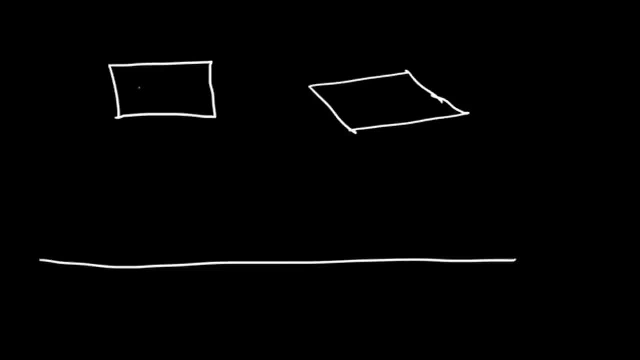 heavier than the flat piece of paper, Let's say it's a 1 kilogram brick. Now, with air resistance, which one will hit the ground? first The brick is going to go straight down, The paper might go this way, then might go that way, and then eventually it will fall to the 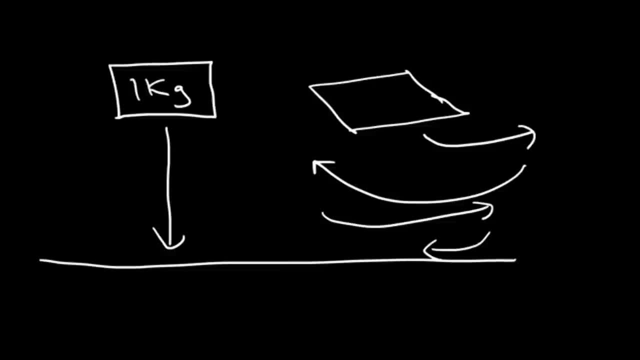 ground because of air resistance. Now what's going to happen if you take the same brick but you crumpled up the paper so that it's very, very small? You take the same paper and crumple it up. Now the effects of air resistance on this. 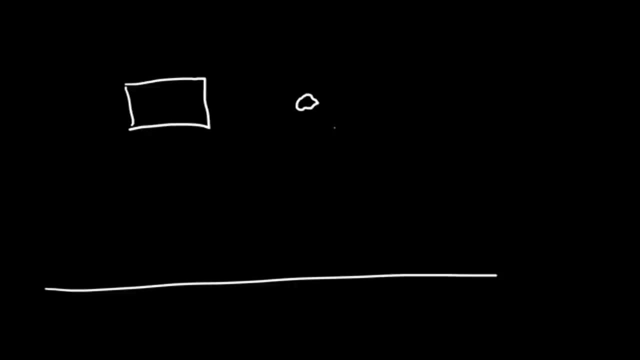 paper will be greatly reduced. If you crumple up the paper very tightly and you let it go, these two will hit the ground approximately about the same time. The greater the surface area of the paper, the greater the effect of air resistance. 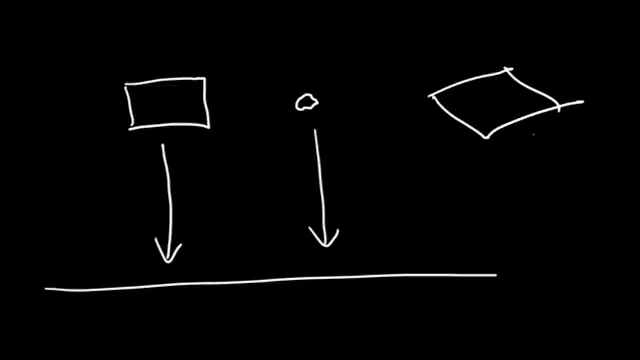 Air resistance increases with surface air. so once you crumple up the paper and then you drop it, you'll see that it's about the same time when it reaches the ground with the brick. The air resistance is greatly reduced. so if you can, 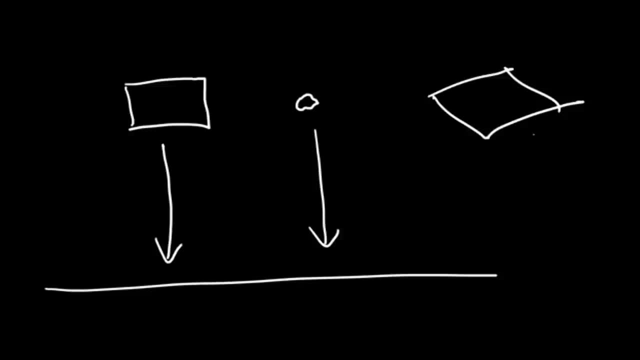 eliminate air resistance completely, then both objects should hit the ground at the exact same time because they're under the influence of the same gravity- Earth's gravitational field. Now let's talk more about the acceleration due to gravity. So if we have a ball and if we 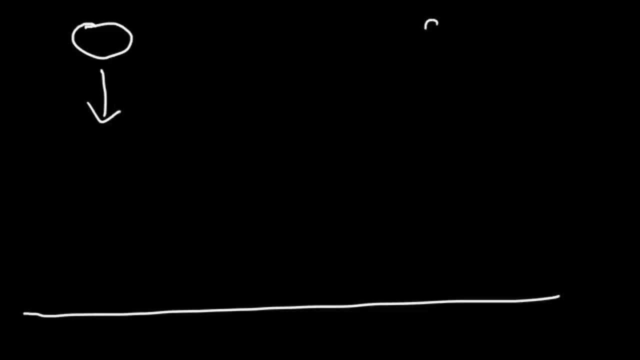 release it from rest. it's going to fall down and it's going to accelerate at the rate of 9.8 meters per second squared. So, if you recall, acceleration tells you how fast the velocity is changing every second. So initially the speed might be. 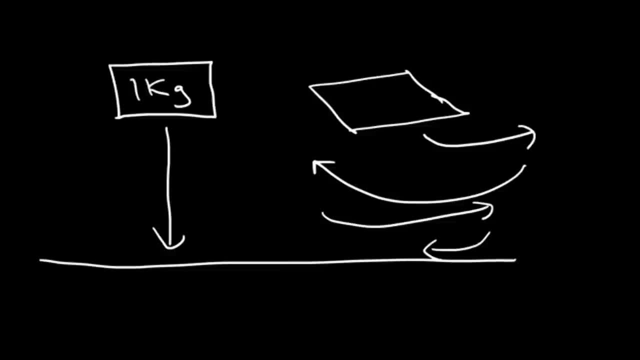 ground because of air resistance. Now what's going to happen if you take the same brick but you crumpled up the paper so that it's very, very small? You take the same paper and crumple it up. Now the effects of air resistance on this. 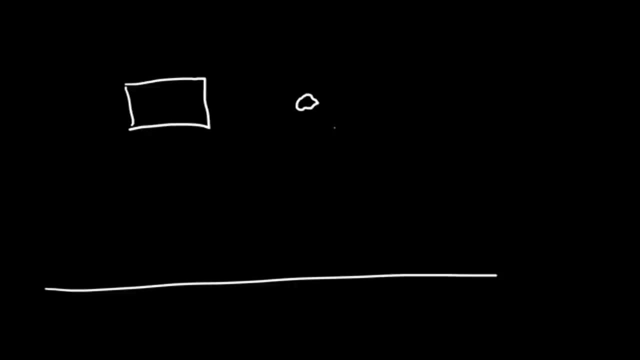 paper will be greatly reduced. If you crumple up the paper very tightly and you let it go, these two will hit the ground approximately about the same time. The greater the surface area of the paper, the greater the effect of air resistance. 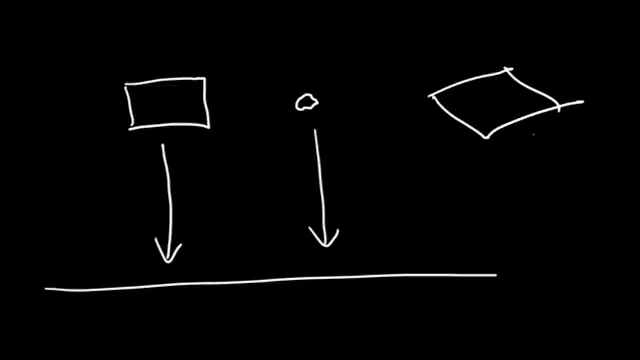 Air resistance increases with surface air. so once you crumple up the paper and then you drop it, you'll see that it's about the same time when it reaches the ground with the brick. The air resistance is greatly reduced. so if you can, 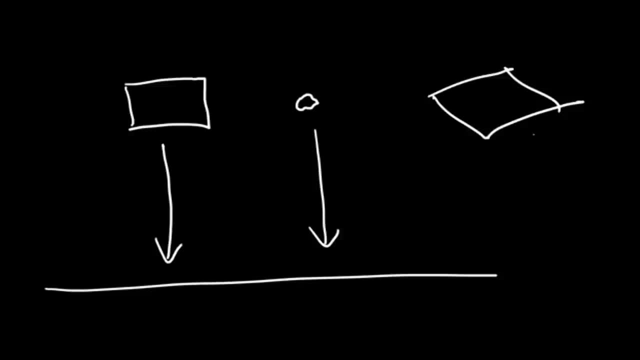 eliminate air resistance completely, then both objects should hit the ground at the exact same time because they're under the influence of the same gravity- Earth's gravitational field. Now let's talk more about the acceleration due to gravity. So if we have a ball and if we 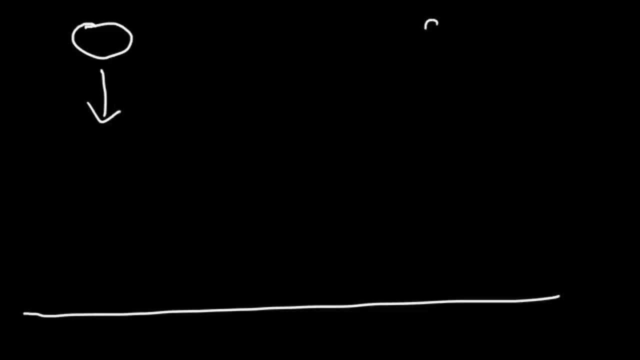 release it from rest. it's going to fall down and it's going to accelerate at the rate of 9.8 meters per second squared. So, if you recall, acceleration tells you how fast the velocity is changing every second. So initially the speed might be. 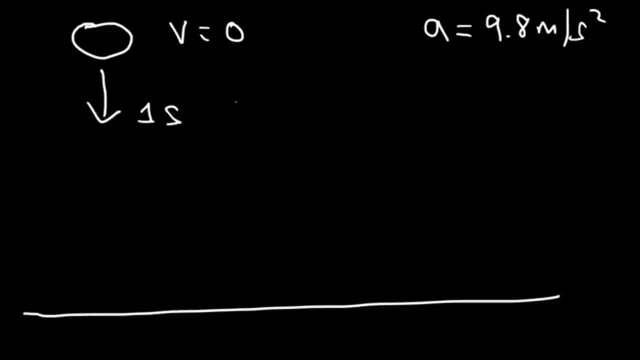 zero. One second later, the velocity is going to be negative: 9.8.. The speed is just positive: 9.8.. Speed is always positive, but velocity can be positive or negative depending on the direction. So because the ball is going in a negative, 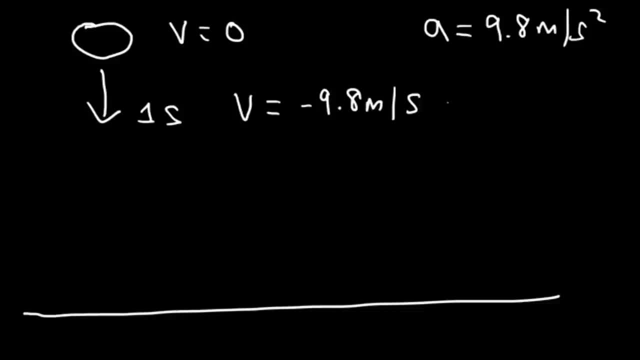 y-direction, the velocity is negative. Now, technically, acceleration is negative: 9.8 meters per second squared. because the object is going to accelerate in the negative y-direction. Gravity pulls things down, not up. Now, two seconds later, the velocity is going to. 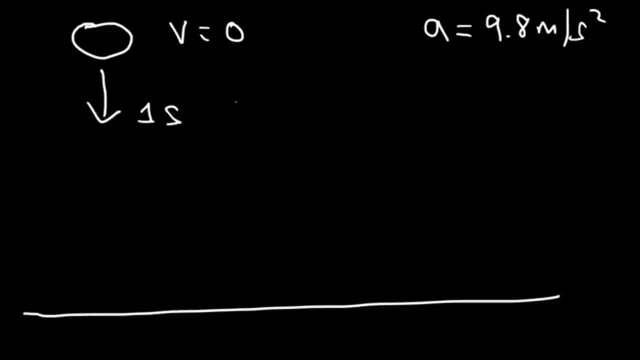 zero. One second later, the velocity is going to be negative: 9.8.. The speed is just positive: 9.8.. Speed is always positive, but velocity can be positive or negative depending on the direction. So because the ball is going in a negative, 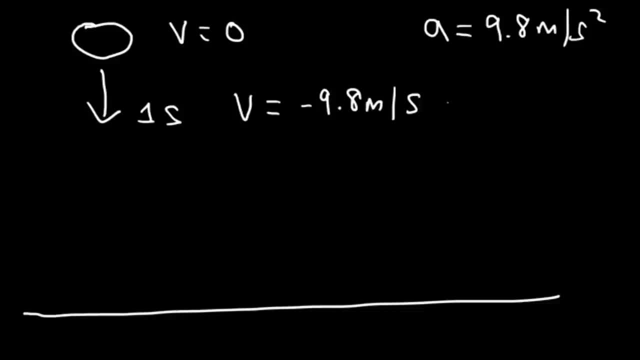 y-direction, the velocity is negative. Now, technically, acceleration is negative: 9.8 meters per second squared. because the object is going to accelerate in the negative y-direction. Gravity pulls things down, not up. Now, two seconds later, the velocity is going to. 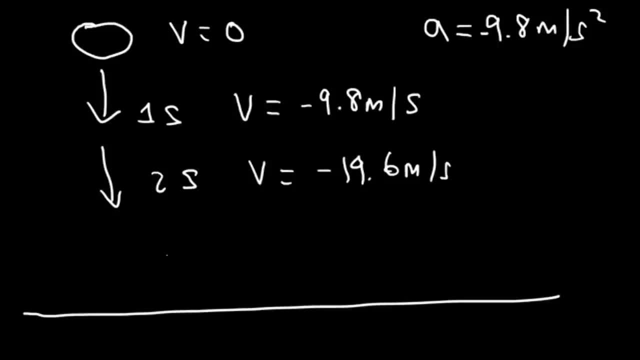 be negative 19.6 meters per second. So every second the velocity is changing. The speed changes. every second The speed changes by 9.8.. So as the ball drops, notice that the velocity is decreasing by 9.8.. It's. 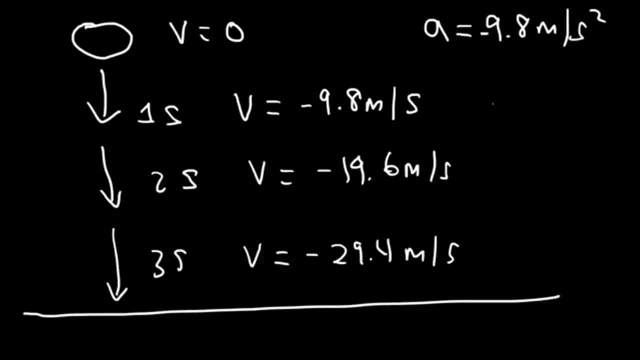 becoming more and more negative. The speed, however, is increasing. Keep in mind, speed is positive. So at this point the speed is positive: 9.8,, it's 19.6, and here it's positive 29.4.. So an object in freefall that's under the influence of 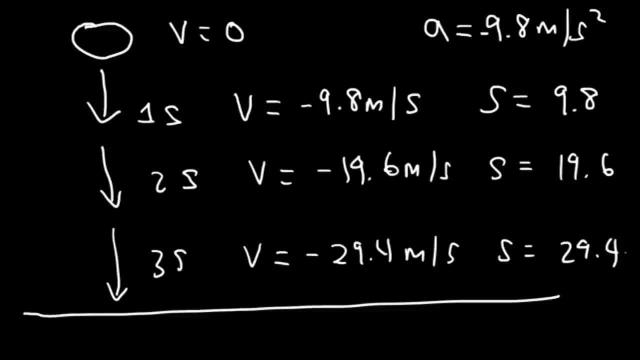 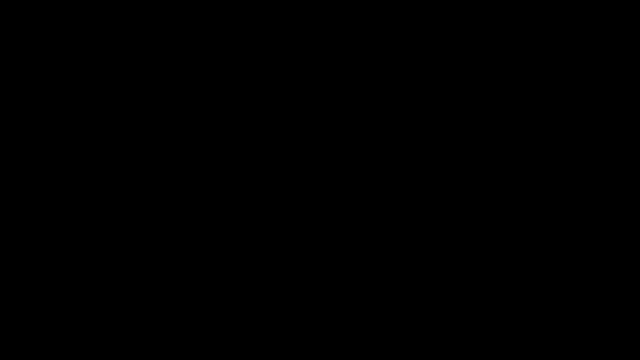 gravity, the speed is increasing by 9.8 every second, but the velocity, because it's negative, is decreasing by 9.8 every second. So remember, acceleration tells you how fast the velocity is changing every second. Now, before we go over a few freefall problems, we need to talk about the 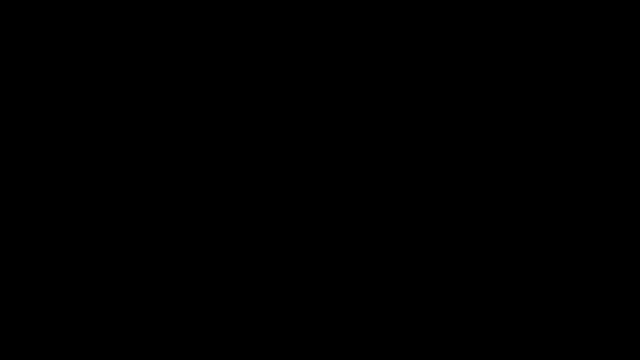 equations that you need to solve them. So, whenever an object is moving with constant speed, this is the equation that you need to use. d is equal to vt. d can be used as distance or displacement. Just remember: distance is a scale of quantity, displacement is a vector. So displacement can be positive or 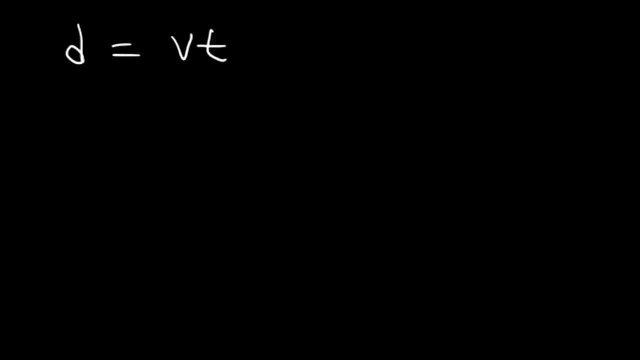 negative, but distance is always positive. So anytime an object is moving with constant speed, you can use this equation. Now, when an object is moving with constant acceleration, you can use any one of these four equations. vfinal is equal to vinitial plus at. 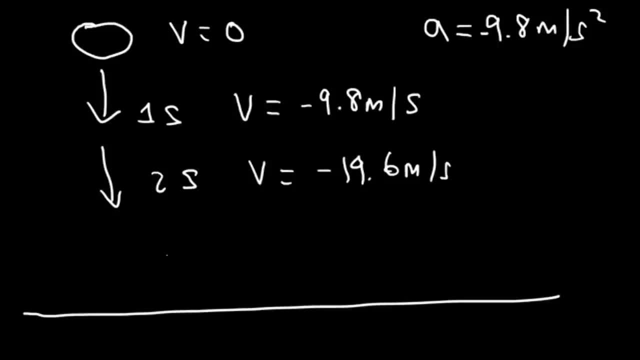 be negative 19.6 meters per second. So every second the velocity is changing. The speed changes. every second The speed changes by 9.8.. So as the ball drops, notice that the velocity is decreasing by 9.8.. It's. 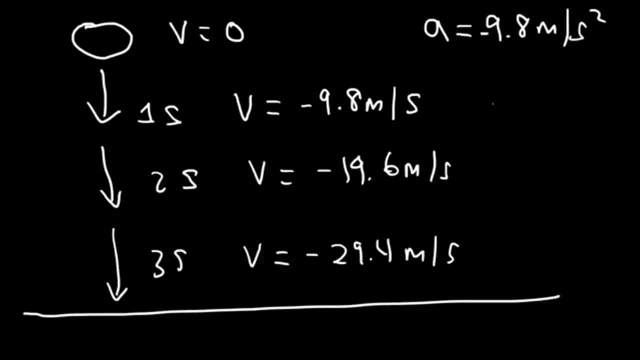 becoming more and more negative. The speed, however, is increasing. Keep in mind, speed is positive. So at this point the speed is positive: 9.8,, it's 19.6, and here it's positive 29.4.. So an object in freefall that's under the influence of 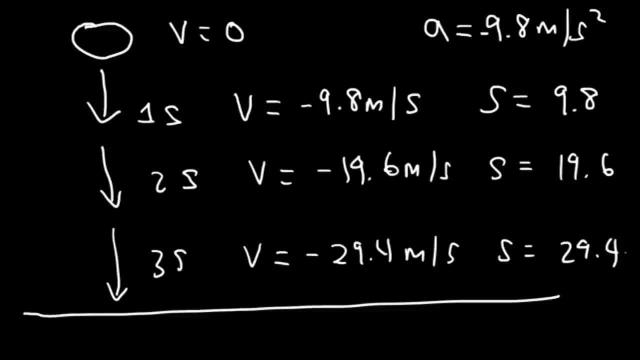 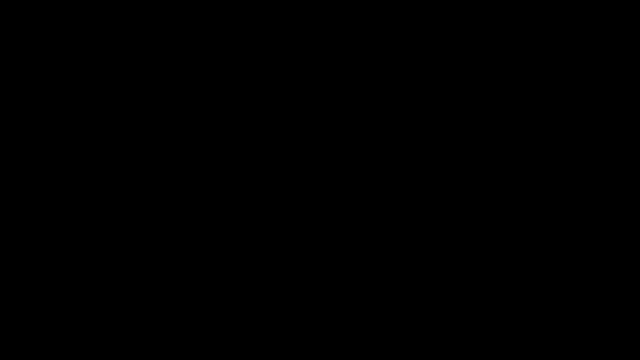 gravity, the speed is increasing by 9.8 every second, But the velocity, because it's negative, is decreasing by 9.8 every second. So remember, acceleration tells you how fast the velocity is changing every second. Now, before we go over a few freefall problems, we need to talk about the 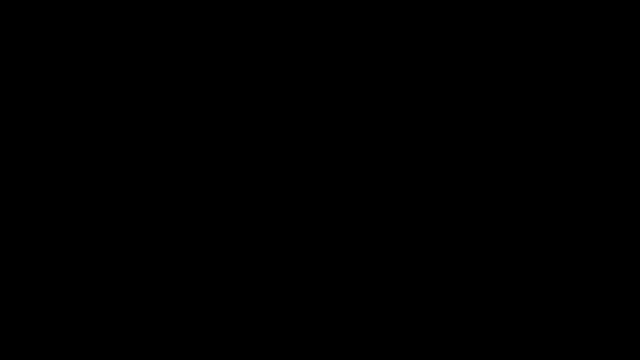 equations that you need to solve them. So, whenever an object is moving with constant speed, this is the equation that you need to use. d is equal to vt. d can be used as distance or displacement. Just remember: distance is a scale of quantity, Displacement is a vector. So displacement can be positive or 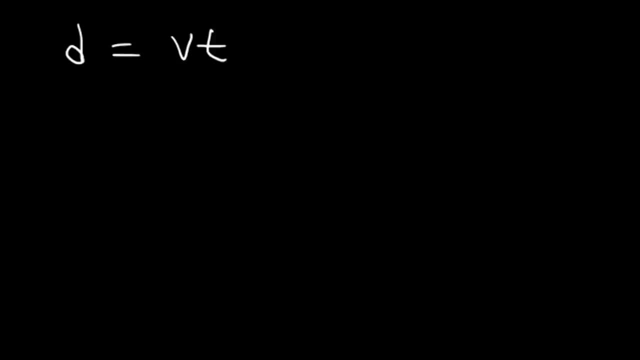 negative, but distance is always positive. So anytime an object is moving with constant speed, you can use this equation. Now, when an object is moving with constant acceleration, you can use any one of these four equations: v final is equal to v initial plus a, t, v. 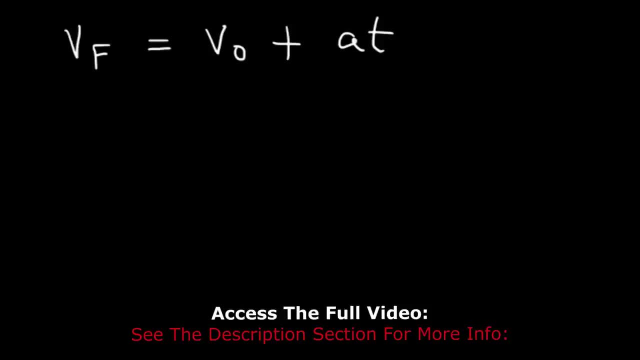 The final can represent the final speed or final velocity. The initial is the initial speed or initial velocity. A is the acceleration, T is the time. So you may see me use the words speed and velocity interchangeably. Just remember that velocity is speed with direction. 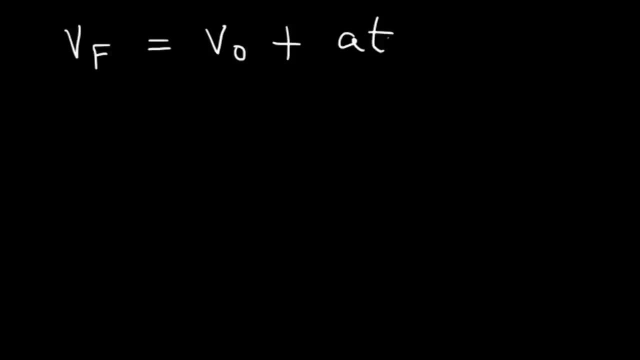 Speed is the scale of quantity. It can only be positive. Velocity can be positive or negative, depending on what direction you're going. So for an object that's moving to the right, the velocity is positive. If the object moves to the left, the velocity is negative. 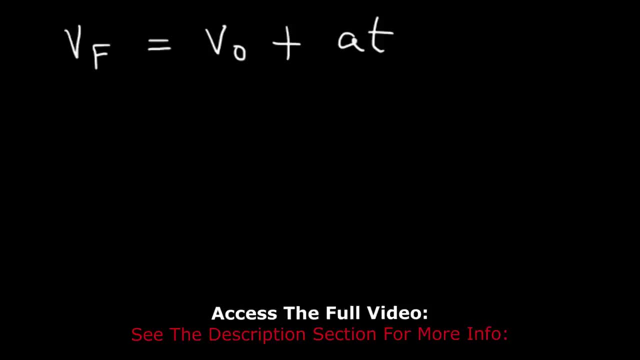 vfinal is equal to vinitial, plus at V final can represent the final speed or final velocity. V initial is the initial speed or initial velocity. A is the acceleration, T is the time. So you may see me use the words speed and velocity interchangeably. 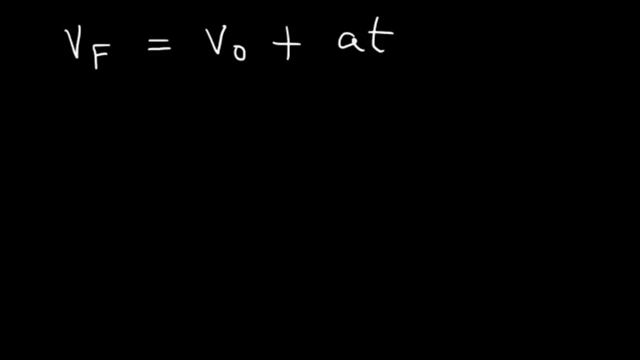 Just remember that velocity is speed. with direction, Speed is the scale of quantity. It can only be positive. Velocity can be positive or negative depending on what direction you're going. So for an object that's moving to the right, the velocity is positive. 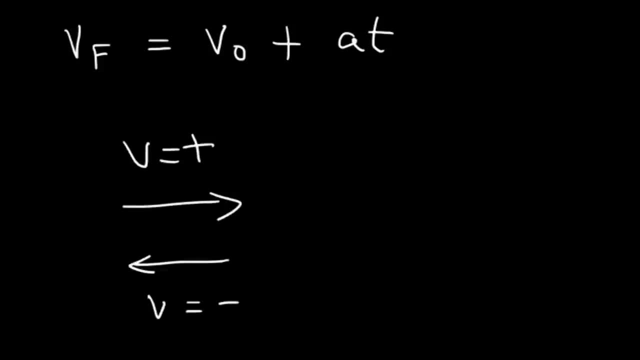 If the object moves to the left, the velocity is negative, But in free fall situations we're dealing with motion in the y direction. When an object goes up, the velocity is positive. When it goes down, the velocity is negative. The next formula that you need to know is: 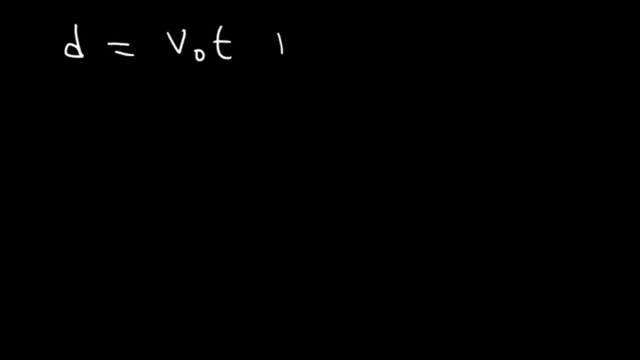 D is equal to V initial T plus 1 half A T squared. And then there's this one: D is equal to 1 half V initial plus V final times T, And V final squared is equal to V initial squared plus 2 A D. 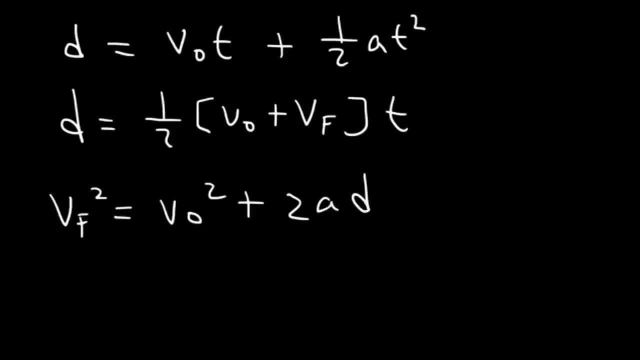 So there are five formulas that you need to know. So these three plus this one And this equation, only when an object is moving at constant speed, When it's moving with constant acceleration, you can use these four equations. So let's start with this problem. 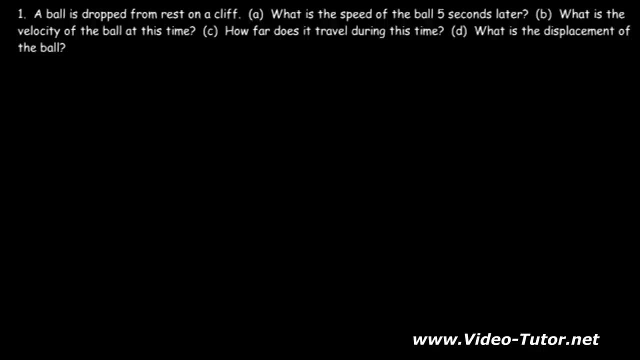 A ball is dropped from rest on a cliff. What is the speed of the ball five seconds later? So let's say: this is the cliff And here is the ball. So it falls down, But we don't know if it's going to fall. 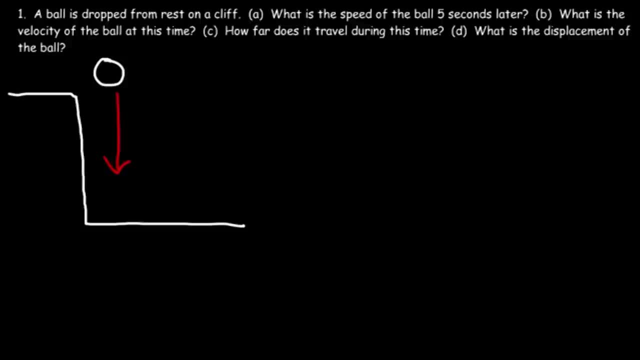 It hits the ground at this point. We just want to find the speed five seconds later. So it's important to make a list of what you have and the variable that you need to find: What is the initial speed of the ball in this problem? 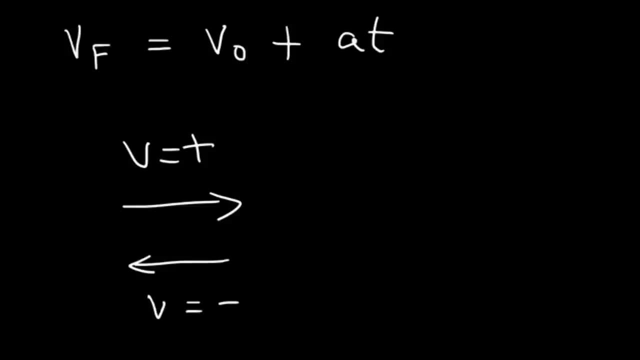 But in free fall situations we're dealing with motion in the Y direction. When an object goes up, the velocity is positive. When it goes down, the velocity is negative. The next formula that you need to know is this one: D is equal to V, initial T plus 1, half A T squared. 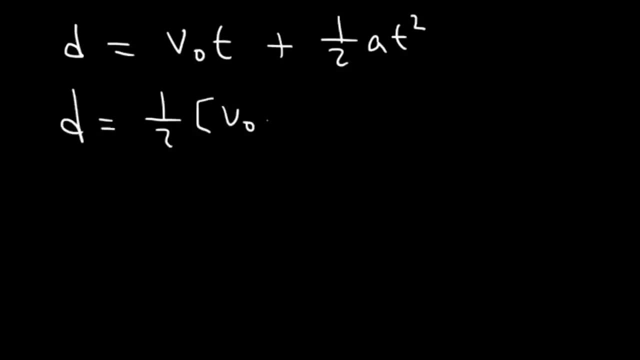 And then there's this one: D is equal to 1 half V initial plus V final times T And V final squared is equal to V initial squared plus 2 A D. So there are five formulas that you need to know. So these three plus this one. 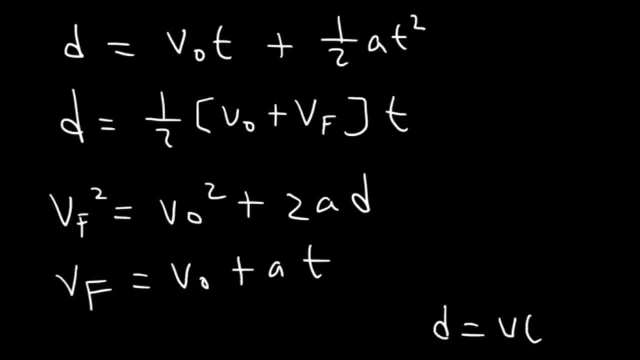 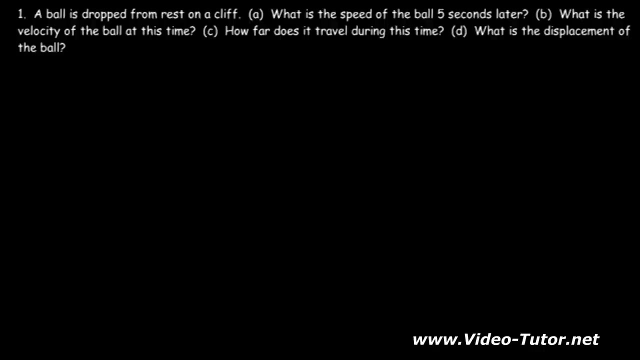 Okay, And this equation only when an object is moving at constant speed, When it's moving with constant acceleration. you can use these four equations. So let's start with this problem. A ball is dropped from rest on a cliff. What is the speed of the ball five seconds later? 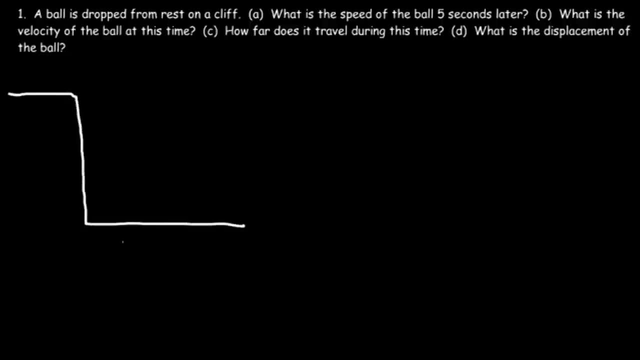 So let's say: this is the cliff And here is the ball, So it falls down, But we don't know if it hits the ground at this point. We just want to find the speed five seconds later. So it's important to make a list of what you have and the variable that you need to find. 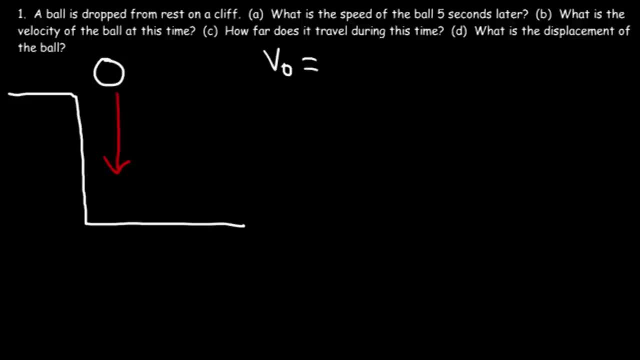 What is the initial speed of the ball? in this problem, Notice that the ball is dropped from rest. So the initial speed is zero. Our goal is to find the final speed. So we're going to find the final speed Now. we know the time. 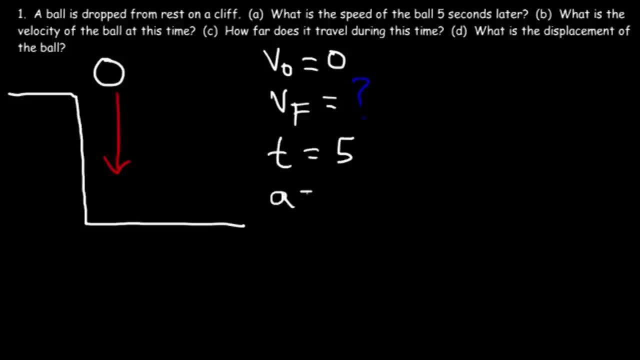 The time is five seconds And the acceleration due to gravity is negative 9.8.. The acceleration due to gravity is in a negative y direction, So that's why it's negative. So what equation that was listed earlier has these four variables? 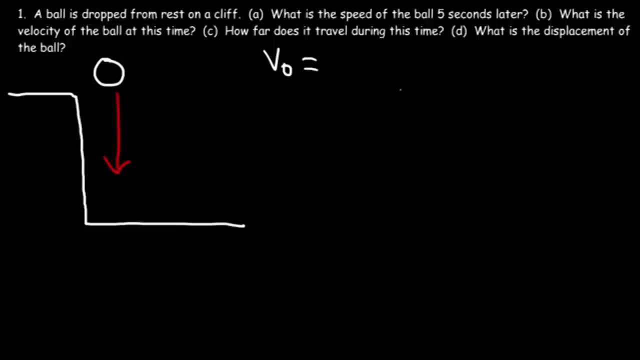 Notice that the ball is dropped from rest. So the initial speed is zero. Our goal is to find the final speed. Now we know the time. The time is five seconds And the acceleration due to gravity is negative 9.8.. The acceleration due to gravity is in a negative y direction. 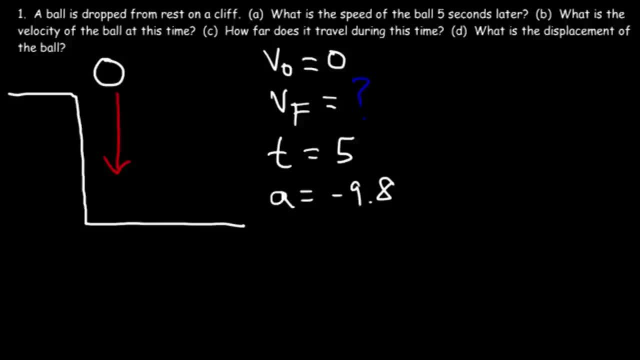 So that's why it's negative. So what equation that was listed earlier has these four variables? The equation that we need is this one: V final is equal to V initial plus AT. V initial is zero. The acceleration is negative 9.8.. 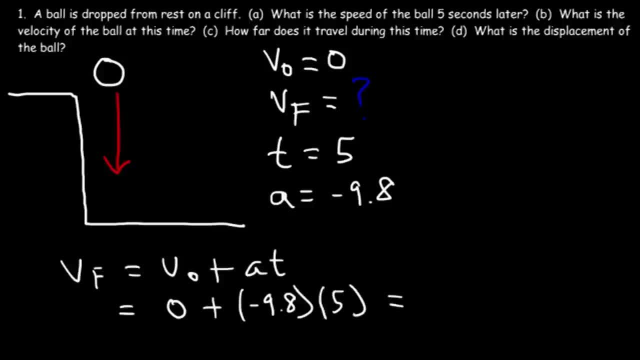 And T is five. So negative 9.8 times five is negative 45. I mean not 45,, but 49.. So now let's go back to the question: What is the speed of the ball five seconds later? Now think about your answer. 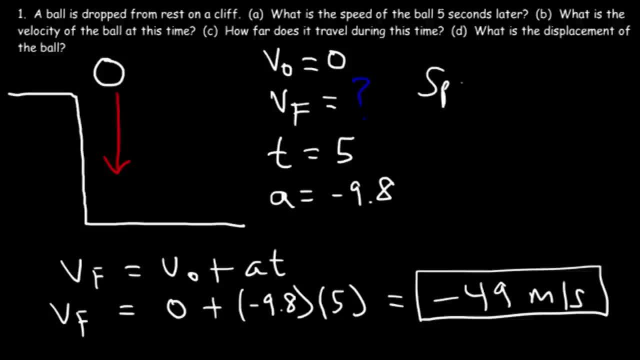 The answer. the speed is positive: 49 meters per second. Remember, speed cannot be negative, So you got to make it positive. So this is the answer for part A. Now part B: what is the velocity of the ball at this time? 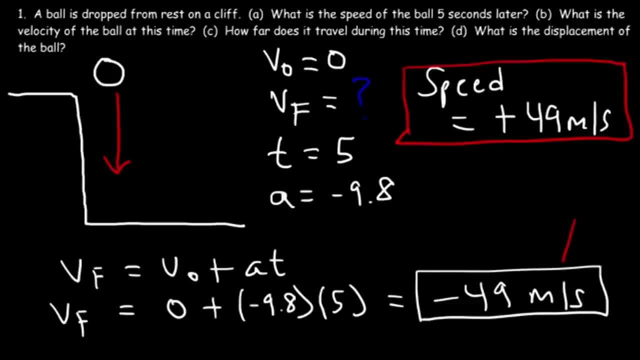 The velocity is negative. So that's the velocity. right there, It's negative 49 meters per second Because the ball is moving in a negative y direction. velocity is negative. Remember, velocity is the vector quantity. Speed is scalar. Now let's move on to part C. 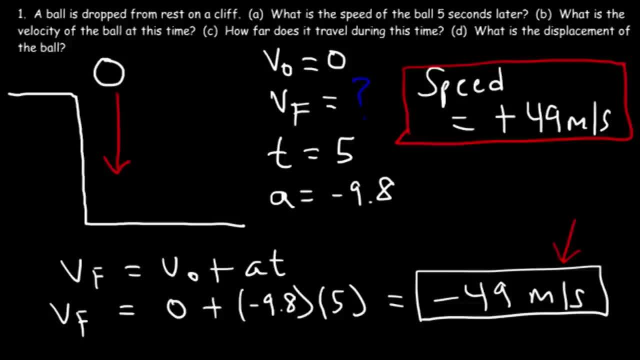 How far does it travel during this time? What equation do you think we need to use? One equation that can help us define it is this one: D is equal to V initial T plus one half AT squared. D is equal to V initial T plus one half AT squared. 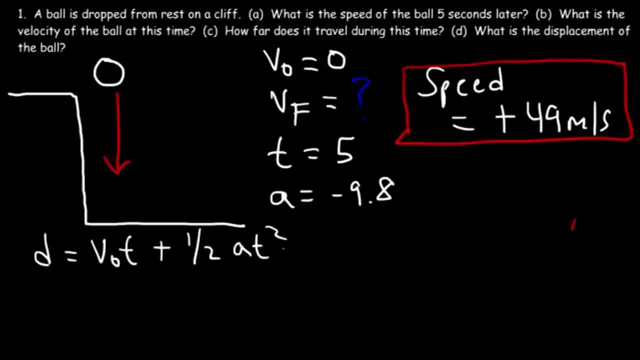 We already have the initial T, We know the initial speed, We know the time And we have the acceleration, So we have enough information to use this equation. So V initial is zero. Zero times T is just going to be zero. Acceleration is negative 9.8.. 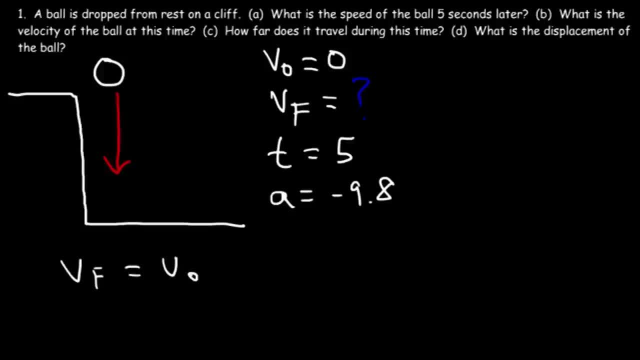 The equation that we need is this one: V final is equal to V initial plus a theta. So what equation is this? V initial is zero, The acceleration is negative 9.8.. And t is five, So negative 9.8 times five is negative 45.. 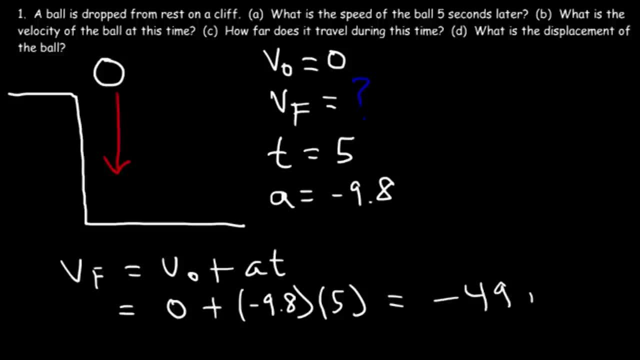 I mean not 45, but 49.. So now let's go back to the question: What is the speed of the ball five seconds later? Now think about your answer. The answer: the speed is positive: 49 meters per second. Remember, speed cannot be negative. 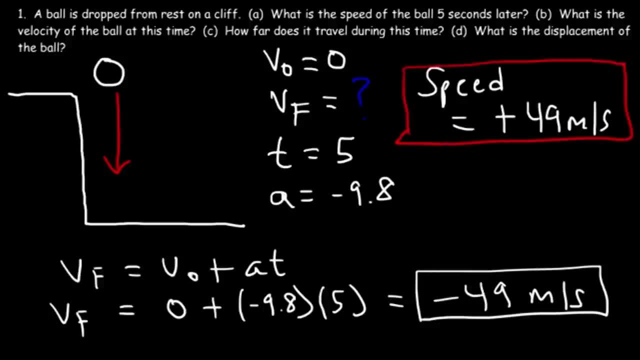 So you got to make it positive. So this is the answer for part a. Now part b. what is the velocity of the ball at this time? The velocity is negative. So that's the velocity right there. It's negative. 49 meters per second. 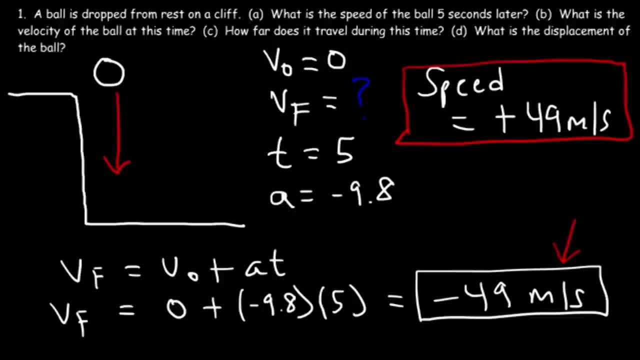 Because the ball is moving in a negative y direction. Velocity is negative. Remember, velocity is a vector. quantity Speed is scalar. Now let's move on to part c. How far does it travel during this time? What equation do you think we need to use? 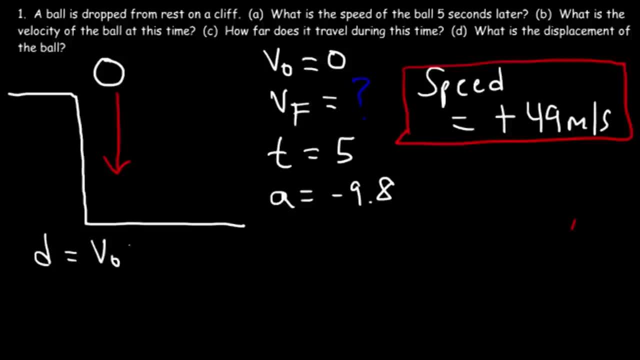 One equation that can help us define it is this one: D is equal to V, initial t plus one half. So this is the velocity of the ball. The velocity is negative. So we can do this: A t squared. We already have the initial speed, we know the time and we have the acceleration. 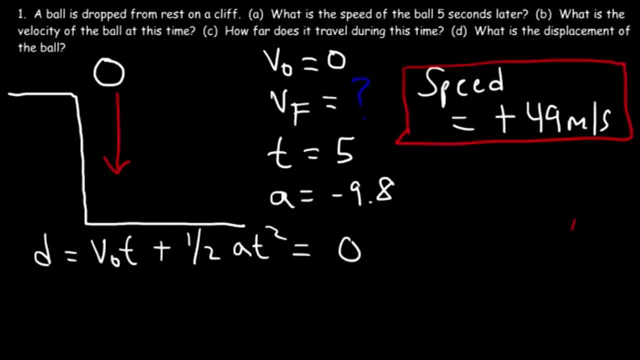 So we have enough information to use this equation. So V: initial is zero, Zero times t is just going to be zero. Acceleration is negative 9.8 and t is five. So half of negative 9.8, that's negative 4.9.. 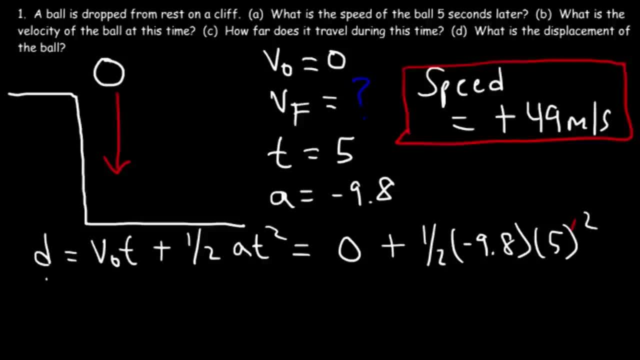 If you multiply that by five squared, That will give you a value of negative 126.99.. point five meters. now what does this answer represent? that answer is not the distance traveled, but rather it's the displacement. this is the answer for part D. remember, displacement is a vector, like velocity. it can be negative or positive. 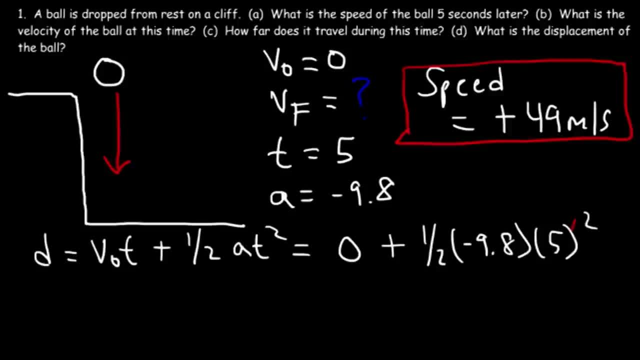 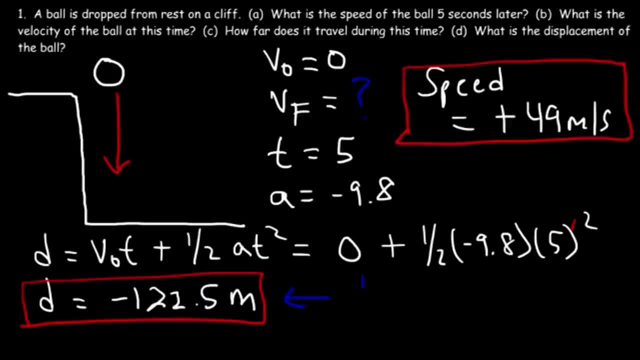 That answer is not the distance traveled, but rather it's the displacement. This is the answer for part D. Remember, displacement is a vector, like velocity, It can be negative or positive. Because the object moves in a negative y direction, the displacement is negative. 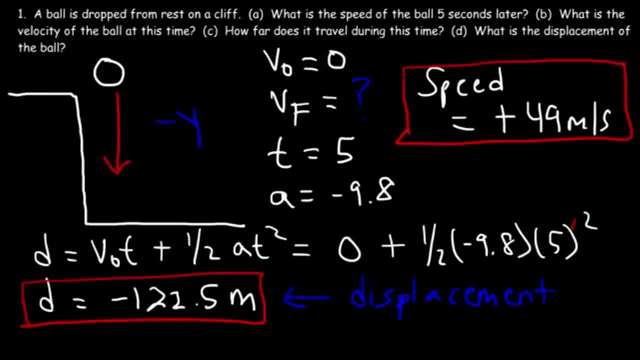 But to answer part C, how far does it travel during this time? Part C is not looking for the displacement, It's looking for the distance traveled. The distance is simply positive, 122.5.. Whenever an object moves in one direction, if it doesn't change direction, if it moves. 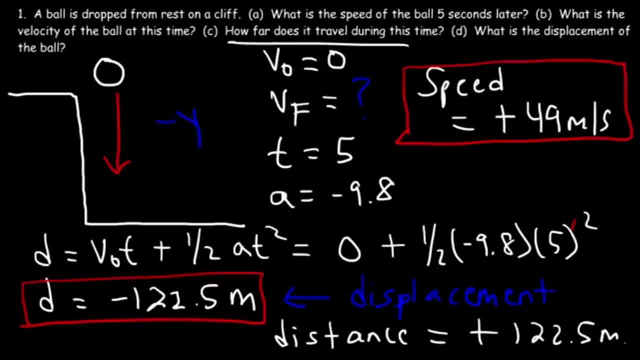 straight. the distance and displacement. they have the same value, They have the same magnitude, but the signs may be different depending on what direction it's going. But anytime you have an object that's moving in a straight line, the distance and displacement. 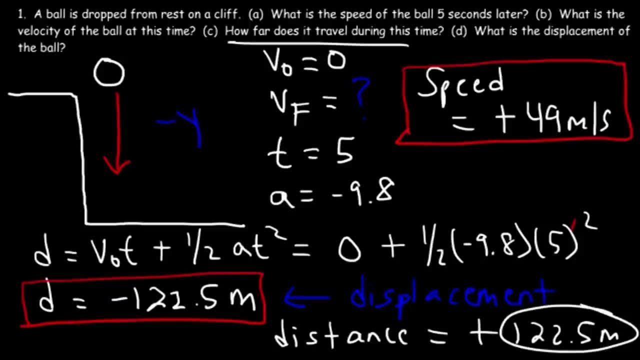 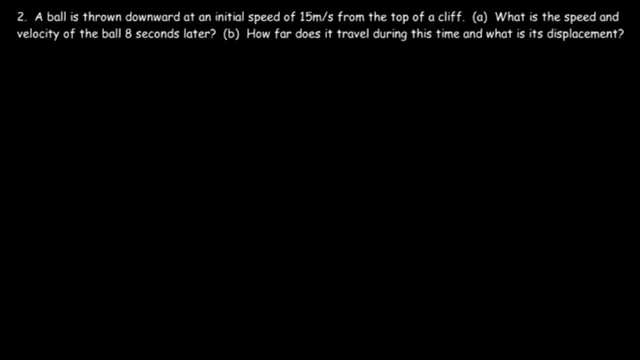 have the same numerical value, Just the signs might be different. So that's it for this problem. Number two: A ball is thrown downward at an initial speed of 15 meters per second from the top of a cliff. What is the speed and velocity of the ball eight seconds later? 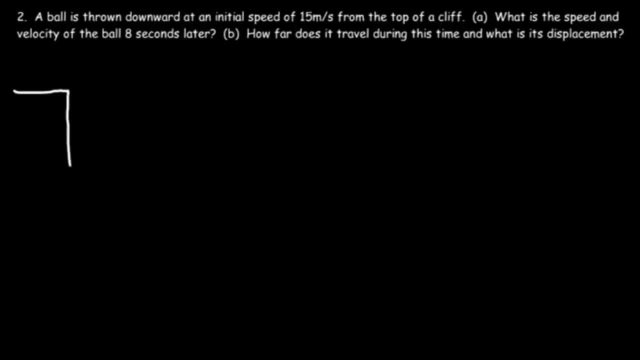 So this problem is similar to the last problem, only one key difference: The ball is not released from rest, Rather, it's thrown down with an initial speed, And that initial speed is 15 meters per second. But let's use the initial velocity when dealing with this equation. 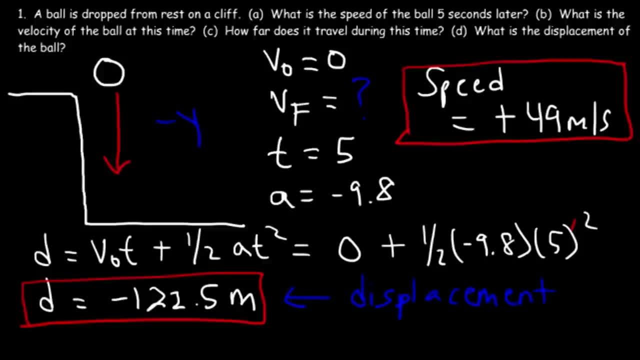 because the object moves in the negative y direction, the displacement is negative. but to answer part C, how far does it travel during this time? part C is not looking for the displacement, it's looking for the distance traveled. the distance is simply positive, 122.5, whenever an object moves in one 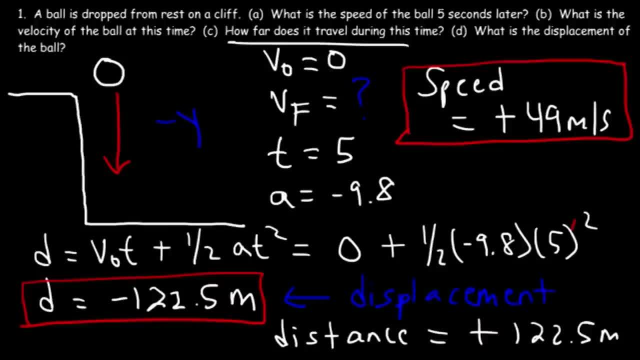 direction if it doesn't change direction, if it moves straight, the distance and displacement they have the same value, they have the same magnitude, but the signs may be different depending on what direction is going. but anytime you have an object that's moving in a straight line, you can't move it in a straight line. you can't move it in a straight line. 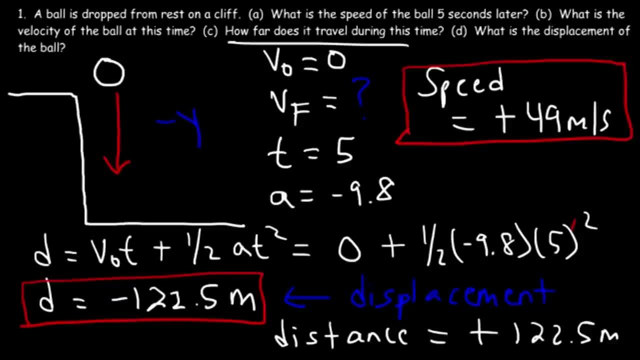 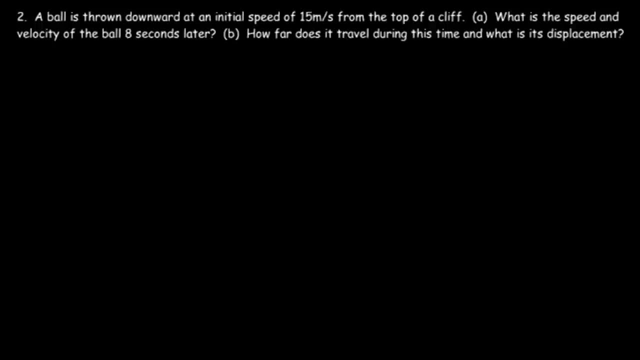 the distance and displacement have the same numerical value, just the signs might be different. so that's it for this problem. number two: a ball is thrown downward at an initial speed of 15 meters per second from the top of a cliff. what is the speed and velocity of the ball eight seconds later? so this: 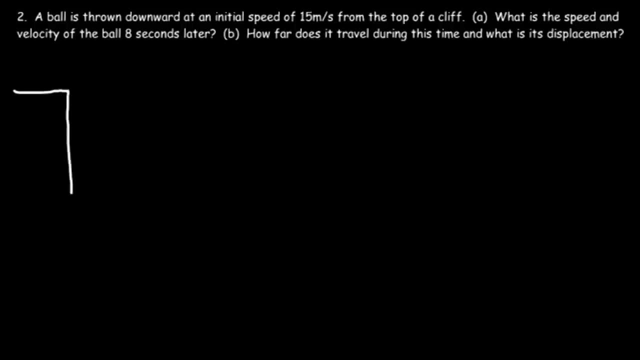 problem is similar to the last problem, only one key difference: the ball is not released from rest, rather, it's throw down with an initial speed, and that initial speed is 15 meters per second. but let's use the initial velocity when dealing with this equation, so we're going to use a. 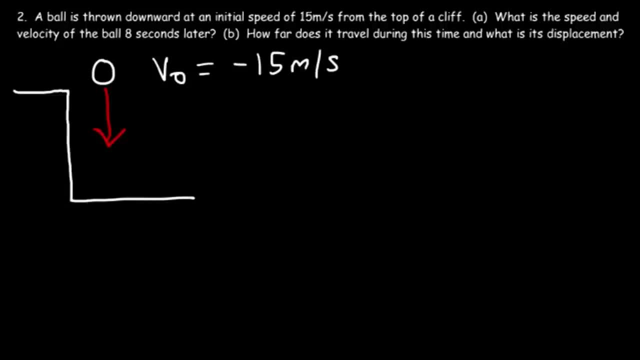 negative 15 meters per second because it's going in a negative y direction. our goal is to find the speed and velocity eight seconds later, so we need to find a final velocity. the time is eight seconds and the acceleration is still negative 9.8, so let's use the same equation to find the final velocity. so 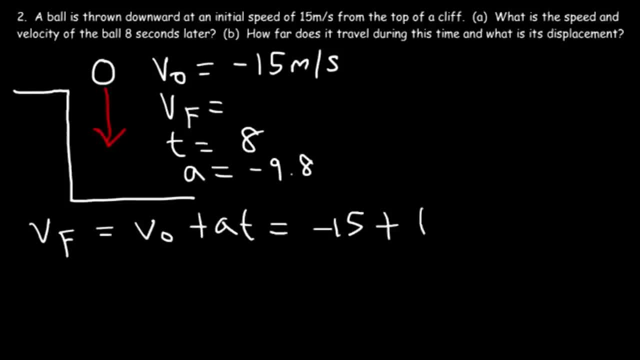 the initial velocity is negative 15 plus the acceleration of negative 9.8, multiplied by the time of eight seconds. negative 9.8 times 8, that's negative 78.4. negative 78.4. so negative 15 plus negative 78.4, that's negative 93.4 meters per second. so this: 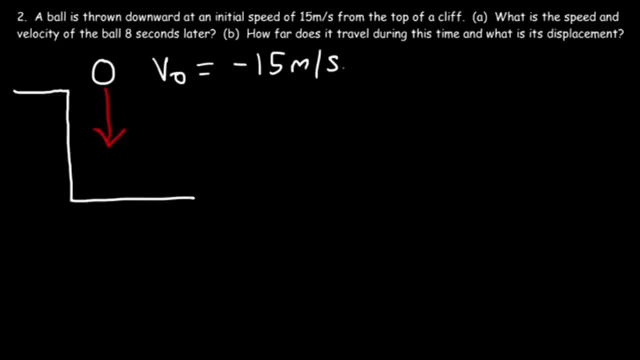 So we're going to use negative 15 meters per second because it's going in the negative y direction. Our goal is to find the speed and velocity eight seconds later. So we need to find the final velocity. The time is eight seconds And the acceleration is still negative 9.8.. 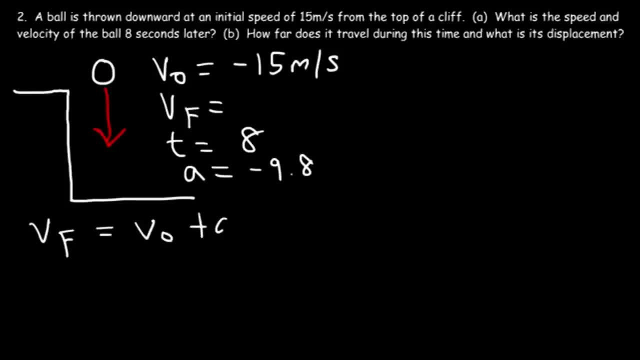 So let's use the same equation to find the final velocity. So the initial velocity is negative 15 plus the acceleration of negative 9.8, multiplied by the time of eight seconds. Negative 9.8 times eight, That's negative 78.4.. 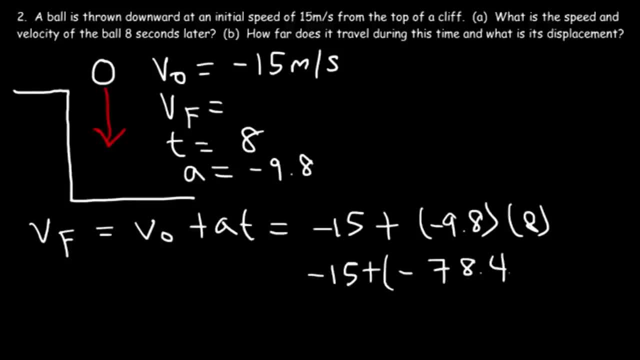 So negative 15.4.. So negative 15 plus negative 78.4, that's negative 93.4 meters per second. So this is the final velocity eight seconds later. The speed eight seconds later is simply positive 93.4.. 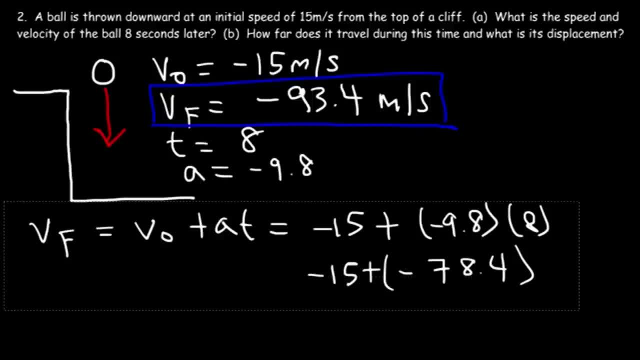 That's it. You just got to change the sign. Just remember It is positive. Now let's find the displacement and also the distance that it travels. So let's use the same equation as the first example. So d is equal to v, initial t, plus one half a t squared. 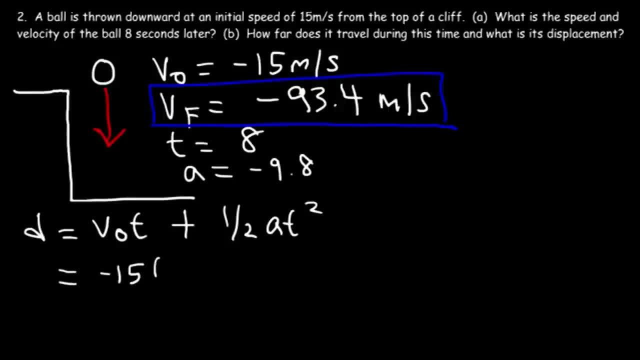 So v initial this time is negative 15.. And t is eight. The acceleration is negative 9.8.. And we're going to plug in eight for t again. So negative 15 times eight, That's negative 120.. Half of negative 9.8 is negative 4.9.. 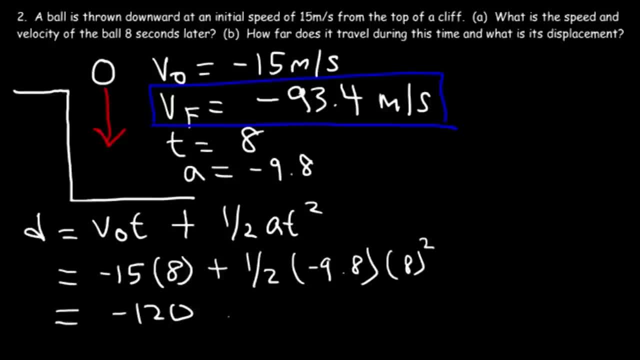 So negative 4.9 times eight squared, That's negative 313.6.. So when adding these two together You should get Negative 433.6 meters. So this is the displacement of the ball during these eight seconds. Now the distance that it travels is positive 433.6 meters. 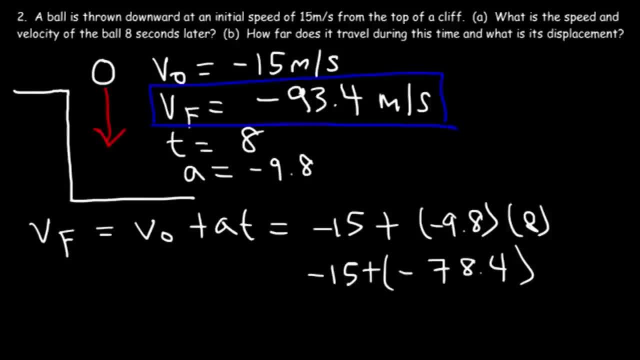 is the final velocity eight seconds later. the speed eight seconds later is simply positive 93.4. that's it. you just got to change the sign. just remember: speed is always positive. now let's find the displacement and also the distance that travels, so let's use 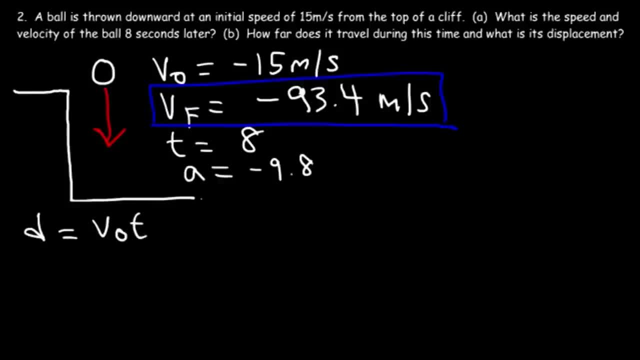 the same equation as the first example. so D is equal to the initial T plus one half 80 squared. so the initial this time is negative 15 and T is a deceleration, is negative 9.8 and we're going to plug in 8 for T. again, it's negative 15 times 8. 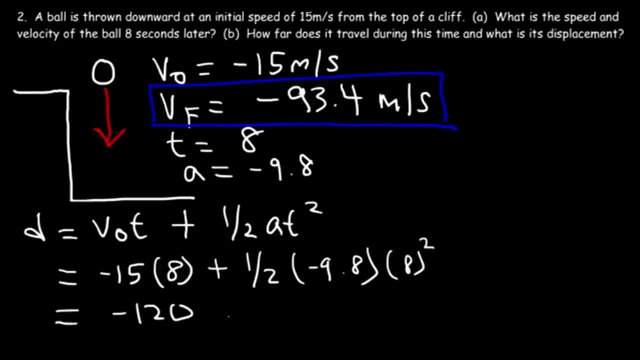 that's negative 120. half of negative 9.8 is negative 4.9. so negative 4.9 times 8 squared that's negative 313.6. so when adding these two together you should get negative 433.6 meters. so this is the displacement of the ball during these. 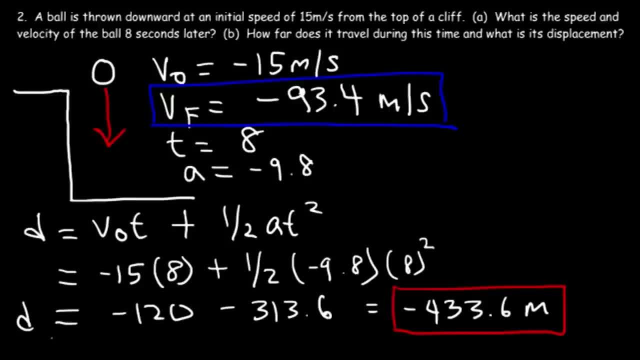 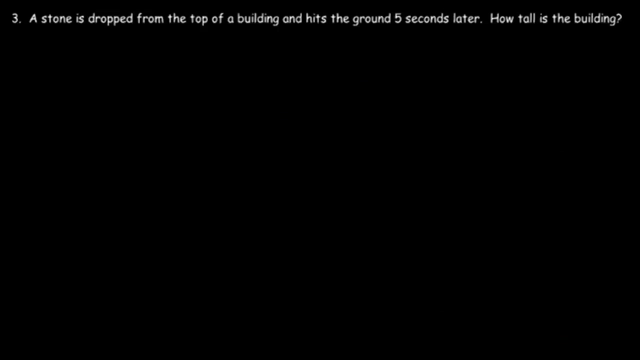 eight seconds. now, the distance that it travels is positive: 433.6 point six meters. so that's the distance that it travels. all you need to do is just make the answer positive. number three: a stone is dropped from the top of the building and hits the ground five seconds later. how tall is the building? 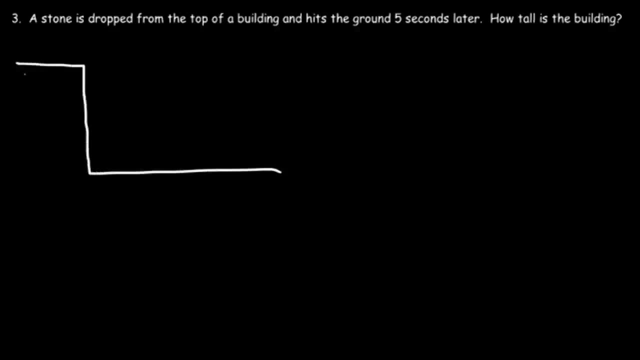 so let's start with a picture. so let's say that's the building and a stone is dropped from the top of a building. our goal is to find the height of the building. the height of the building is basically the distance that the ball travels until it hits the ground. so if we could find the distance. 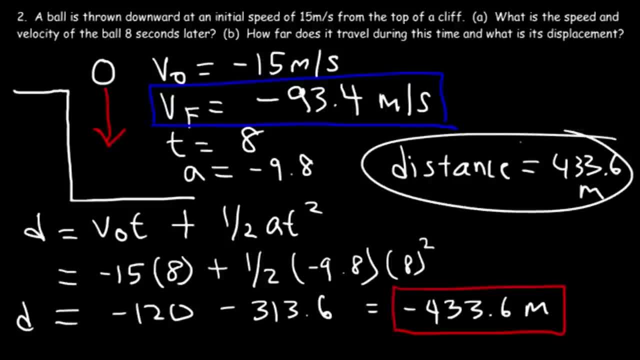 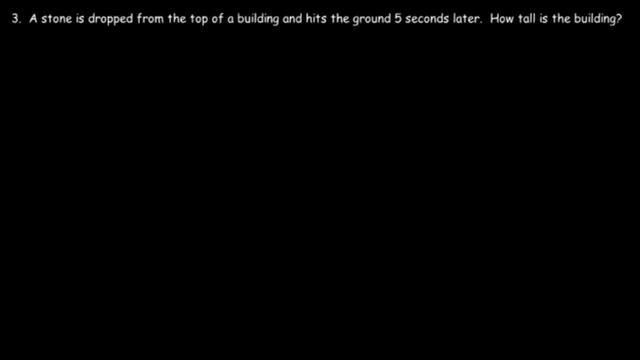 So that's the distance that it travels. All you need to do is just make the answer positive. Number three: A stone is dropped from the top of the building and hits the ground five seconds later. How tall is the building? So let's start with a picture. 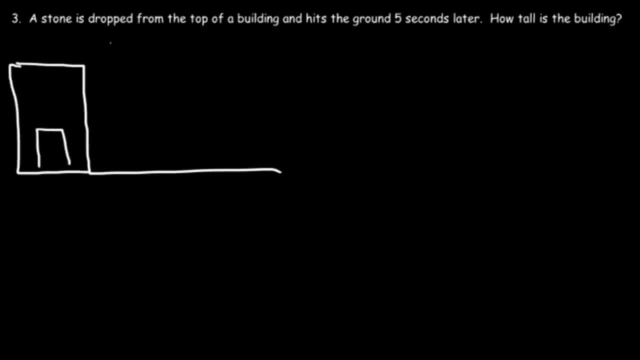 So let's say that's the building And a stone is dropped from the top of the building. Our goal is to find The height of the building. The height of the building Is negative. The height of the building is basically the distance that the ball travels until it hits the ground. 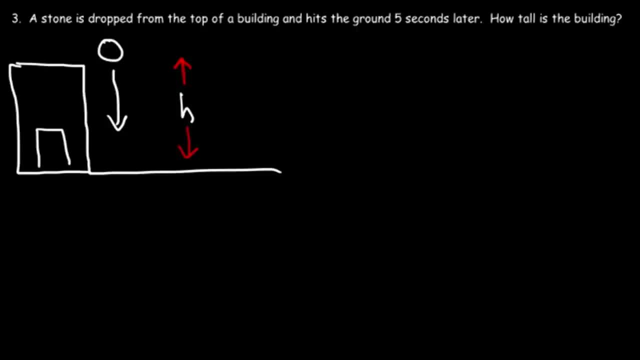 So if we could find the distance that it travels, we could find the height of the building. Now, what equation should we use? In order to find out which equation to use, we need to make a list of everything that we have. 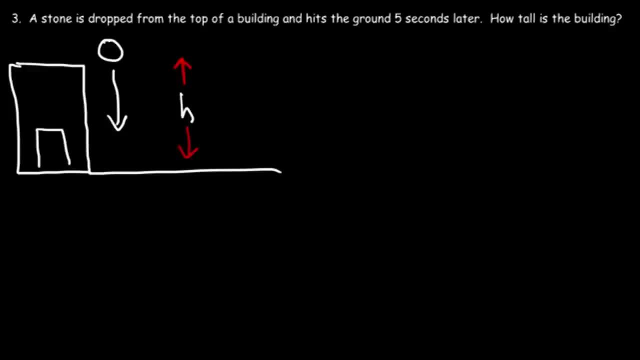 Now it didn't say the stone is thrown down. So therefore, if the stone is dropped from the top of a building, we know it's dropped from rest, which means the initial speed is zero. We don't know what the final speed is, but we do have the time and we know the acceleration. 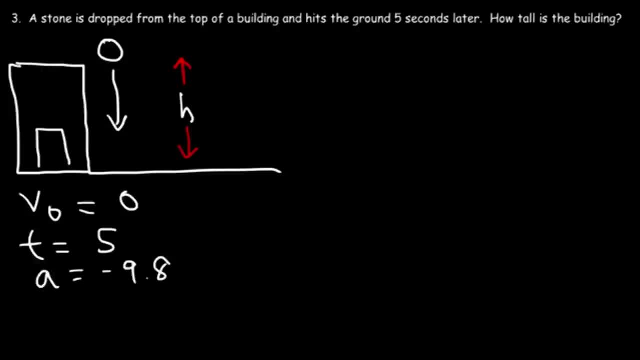 For any object in free fall, any object that's fallen under the influence of gravity, this acceleration will always be the same value in the y direction. So our goal is to find d In the y direction, which is the same as the height. 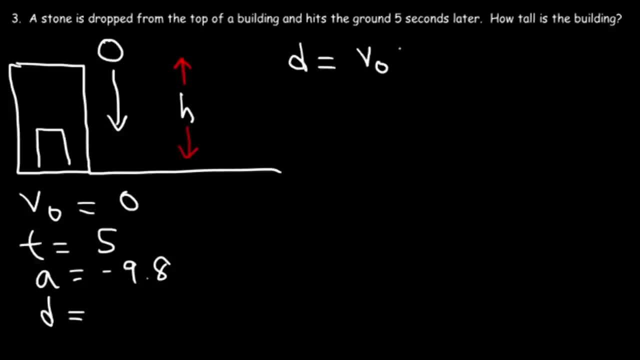 So once again we could use this equation: d is equal to v initial, t plus one half a t squared. But because v initial is zero, we don't need this portion of the equation. So therefore, the height of the building which we can replace with the displacement, the height of the building is going to be just one half a t squared. 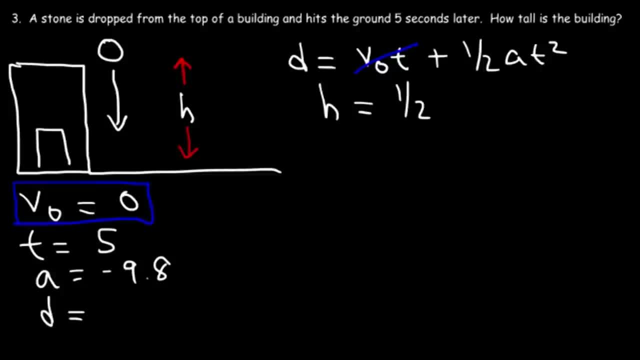 For those of you who just want a simple formula to find this answer, But I'm going to use d in this example. a is negative 9.8.. t is 5.. So negative 4.9, which is half of 9.8, times 5 squared. 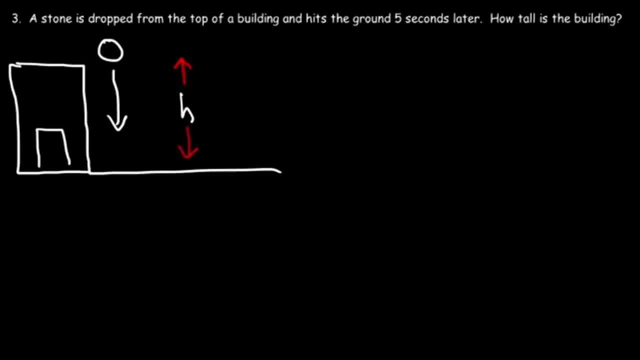 that it travels. we could find the height of the building. now what equation should we use? in order to find out which equation to use, we need to make a list of everything that we have now. it didn't say the stone is thrown down, so therefore, if the stone is dropped from the top of a building, we know it's. 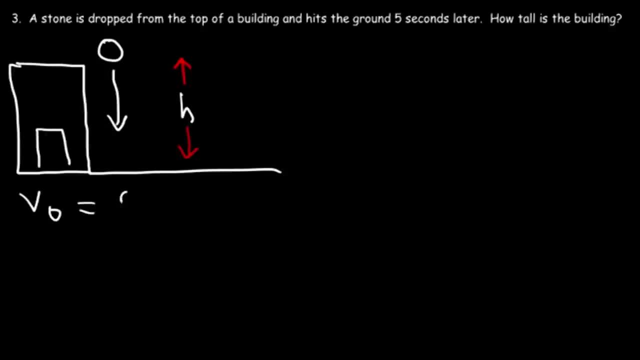 dropped from rest, which means the initial speed is zero. we don't know what the final speed is, but we do have the time and we know the acceleration for any object in freefall and the object that's fallen under the influence of gravity. this acceleration will always be the same value in the y-direction. so our 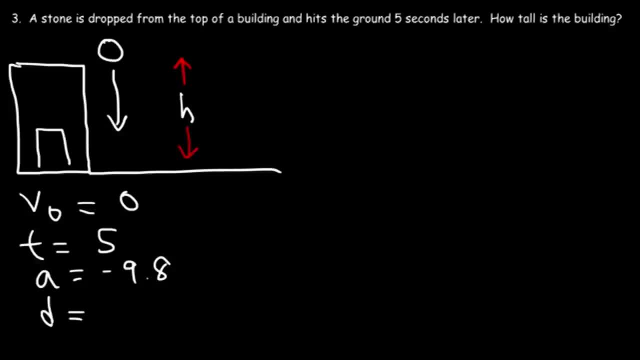 goal is to find D in the y-direction, which is the same as the height. so once again we could use this equation: d is equal to the initial t plus one-half 80 square, but because the initial is 0, we don't need this portion of the equation. 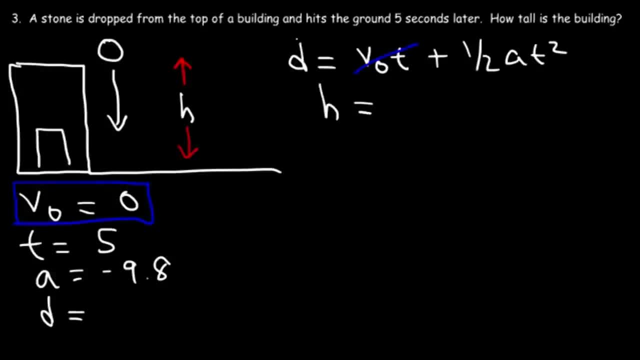 so, therefore, the height of the building which we can replace with the displacement, the height of the building, is going to be just one half 80 squared. for those of you who just want a simple formula to find this answer, I'm going to use D. in this example, a is negative 9.8, t is 5, so negative 4.9. 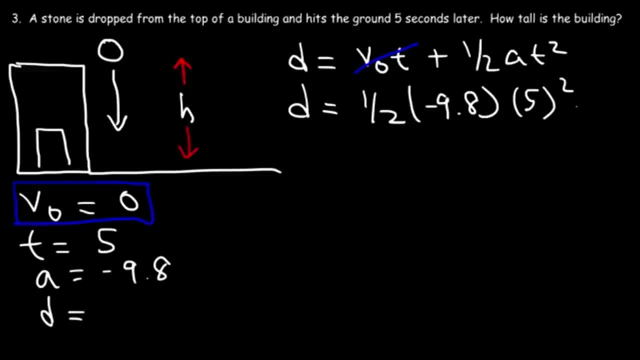 which is half 9.8 times 5 squared, that's negative 122.5 meters. so keep in mind that's the displacement of the ball. so what that means is that the ball travels a hundred and 22.5 meters down before hits the ground. so 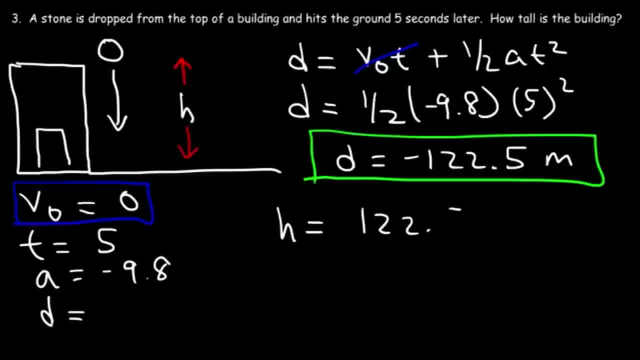 therefore, the height of the building is the same. but you don't need to describe the height of the building using a negative number. all you need to say is is that on the building is a hundred and twenty-two point five meters tall. you don't have to say negative 122.5, that's not going to. 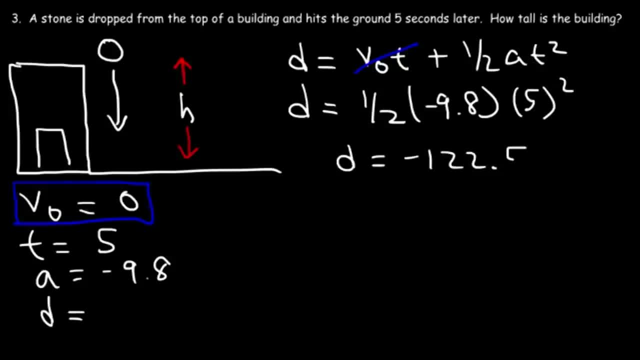 That's negative 122.5 meters. So keep in mind that's the displacement of the ball. So what that means is that the ball travels 120.. 122.5 meters down before it hits the ground. So therefore the height of the building is the same. 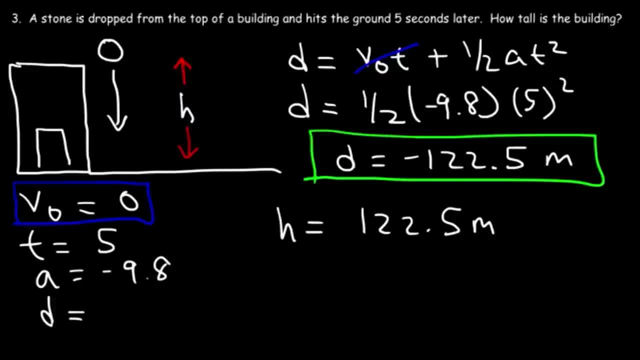 But you don't need to describe the height of the building using a negative number. All you need to say is that the building is 122.5 meters tall. You don't have to say negative 122.5.. That's not going to make any sense. 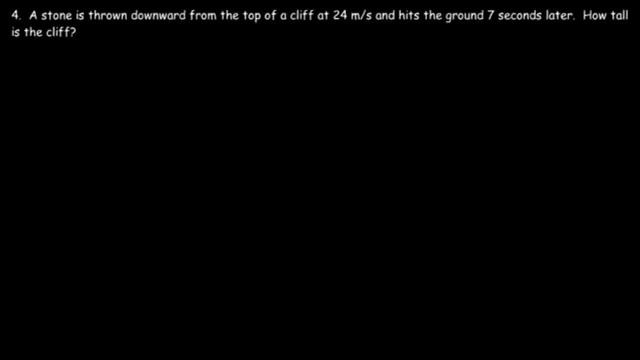 So this is the height of the building. So now that you know how to do the last problem, Go ahead and do the next problem. Go ahead and try this one. A stone is thrown downward from the top of a cliff at 24 meters per second. 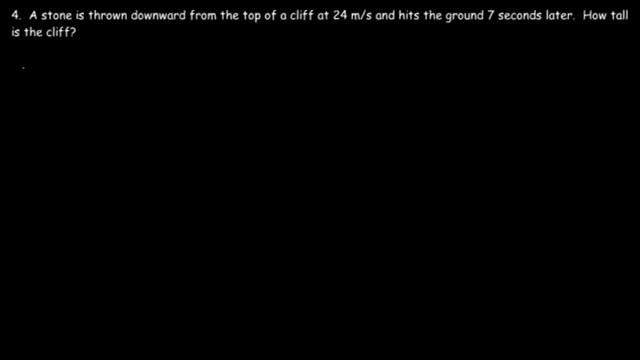 And hits the ground 7 seconds later. How tall is the cliff? So it's no longer released from rest, But someone just throws it down. So, therefore, we know that there is an initial speed, which is 24.. 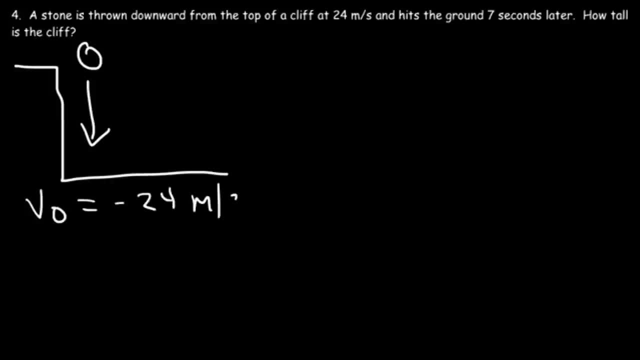 But we're going to use the initial velocity, which is negative: 24 meters per second. We have the time it takes for it to hit the ground, That's 7 seconds. The acceleration in the y direction is still negative: 9.8 meters per second. squared. 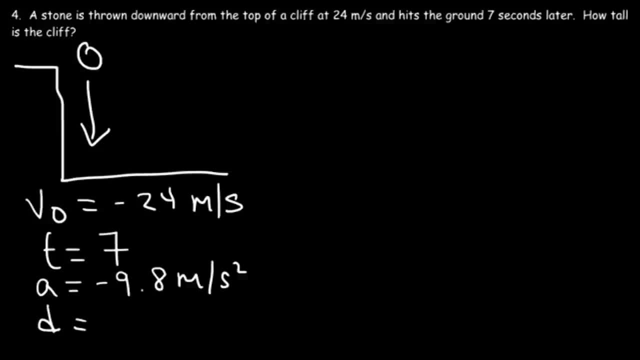 Our goal is to find the height of the cliff, So basically we just need to find the displacement of the ball. So let's use the same formula. D is equal to V initial T plus 1 half A T squared. This time we need this portion of the equation. 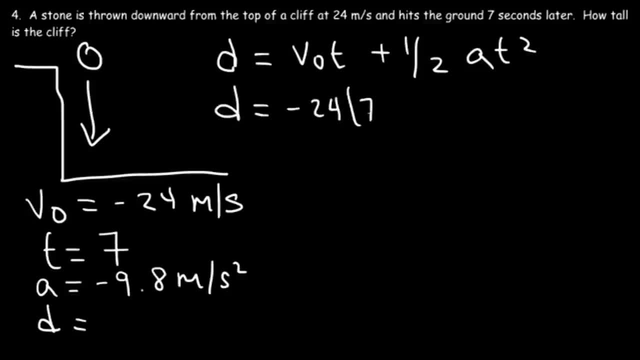 So V initial is V. initial is negative 24.. T is 7.. A is the same. And now let's go ahead and find the answer: Negative 24 times 7. That's negative 168.. And negative 4.9 times 7 squared. 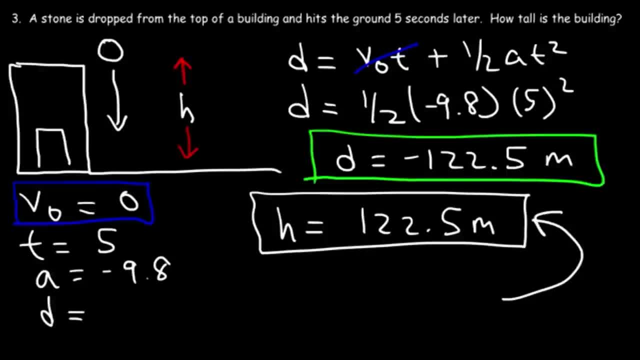 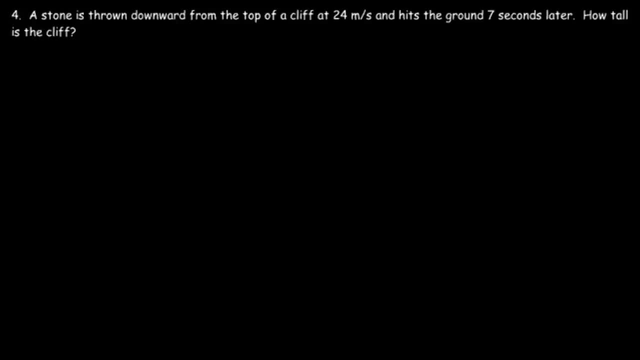 make any sense. so this is the height of the building. so now that you know how to do the last problem, go ahead and try this one. a stone is thrown downward from the top of a cliff at 24 meters per second and hits the ground seven seconds later. 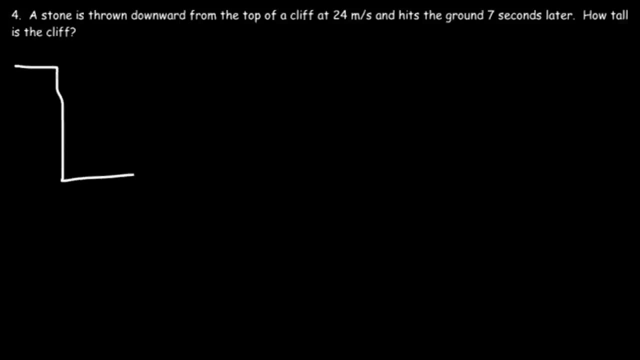 how tall is the cliff? so to no longer release from rest, but someone just throws it down. so therefore, we know that this is an initial speed, which is 24. we're going to use the initial velocity, which is negative 24 meters per second. we have the time it takes for it to hit the ground, that seven seconds. the 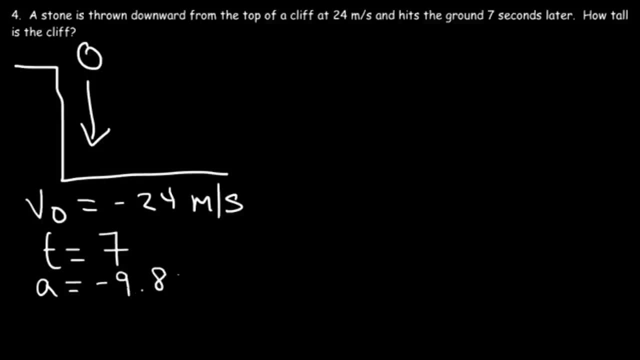 acceleration in the y direction is still negative: 9.8 meters per second squared. our goal is to find the height of the cliff. it's basically we just need to find the displacement of the ball. so let's use the same formula. d is equal to the initial t plus one-half a t squared. this: 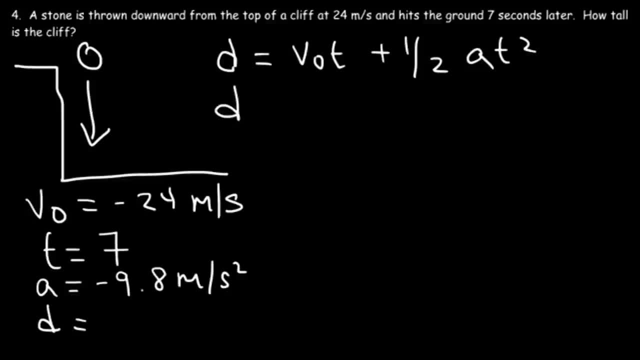 time we need this portion of the equation. so the initial is negative 24, t is 7a is the same. and now let's go ahead and find the answer. negative 24 times 7, that's negative 168, and negative four point nine times seven squared, that's about negative 240.1. so the displacement of 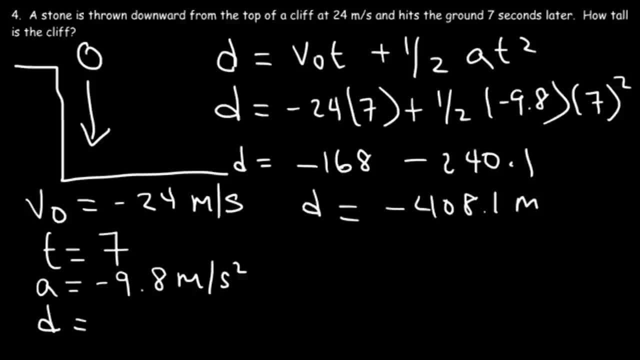 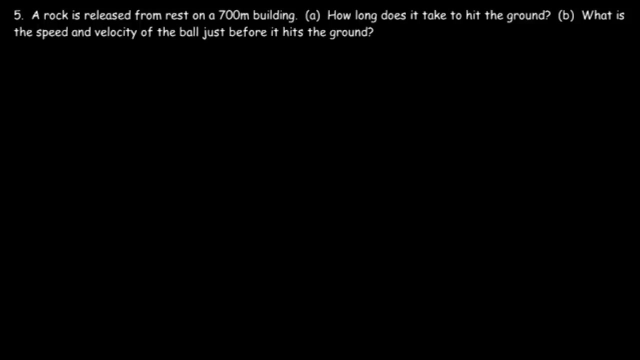 the ball is negative 408.1 meters. so what this means is that the ball travels 408.1 meters in a negative y direction. that's why it's negative. but the distance traveled, which is the height of the cliff, that's positive 408.1 meters, and that's the answer. a rock is released from rest. 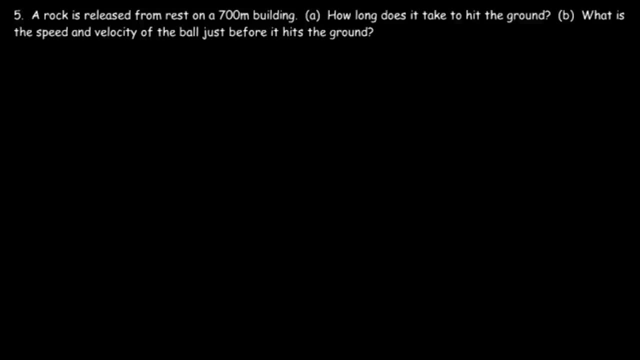 on a 700 meter building, how long does it take to hit the ground? what is the speed and velocity of the ball just before it hits the ground? well, let's start with a picture. so this time we're given the height of the building and initially we need to find out how long does it take to hit the ground. so 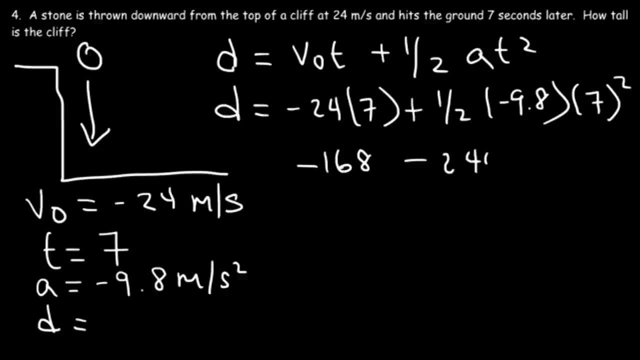 That's about negative 240.1.. So the displacement of the ball is negative 408.1 meters. So what this means is that the ball travels 408.1 meters in a negative y direction. That's why it's negative. 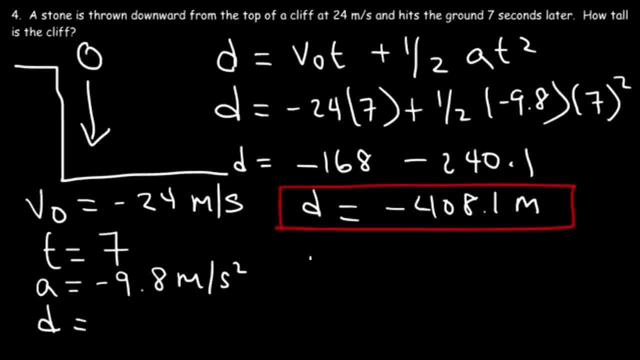 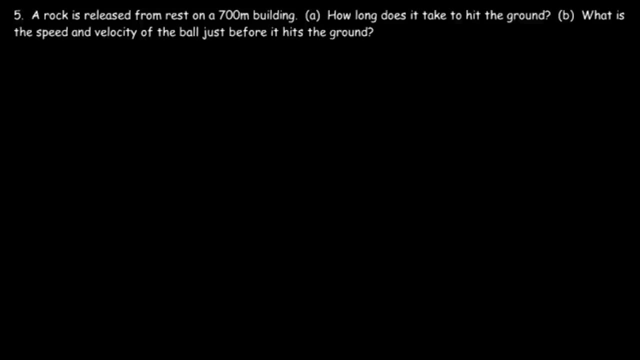 But the distance traveled, which is the height of the cliff, that's positive 408.1 meters, And that's the answer. A rock is released from. A rock is released from rest on a 700-meter building. How long does it take to hit the ground? 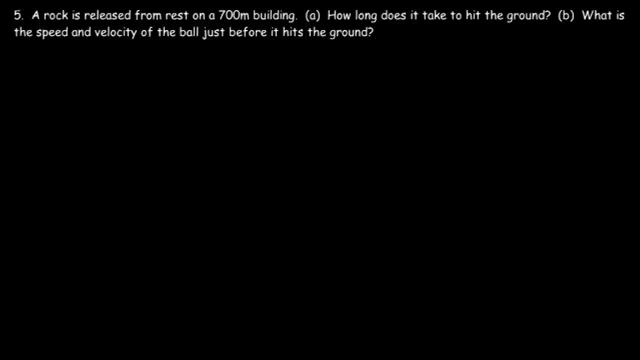 What is the speed and velocity of the ball just before it hits the ground? Well, let's start with a picture. So this time we're given the height of the building And initially we need to find out how long does it take to hit the ground. 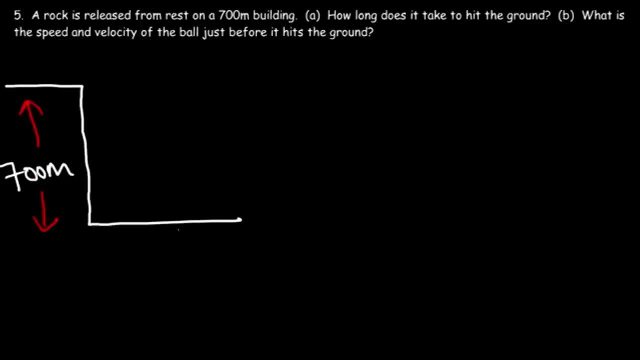 So we've got to find the time. Let's make a list of what we have. The rock is released from rest, So the initial The speed is zero. We have the acceleration in the y direction, That's negative 9.8.. 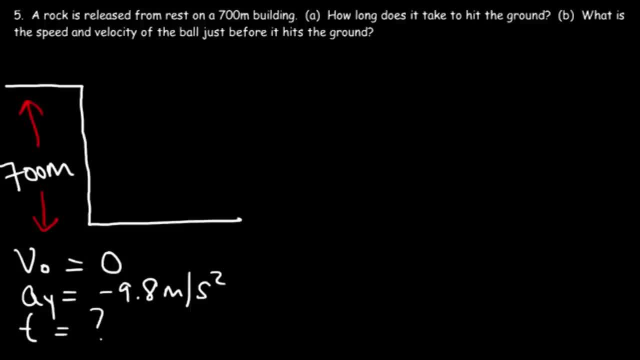 We're looking for the time, But we do have the displacement. The displacement in the y direction is not positive 700, but it's negative 700. Because the ball is moving in the negative y direction. So let's use this: 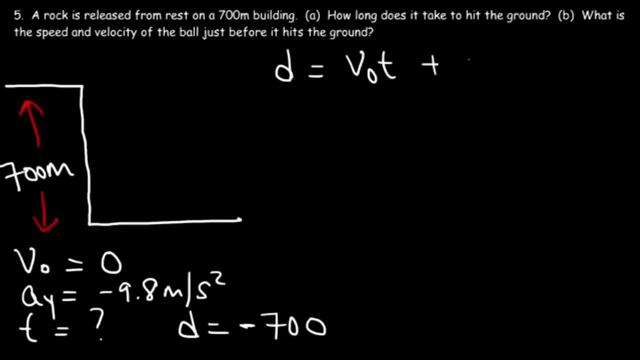 D is equal to V initial t plus one-half a t. squared, Now d is negative 700.. V initial, fortunately, is zero, So we can avoid using the quadratic equation. The acceleration is negative 9.8.. So now all we've got to do is find t. 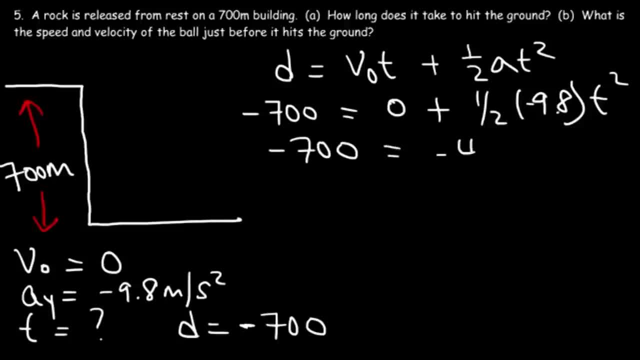 So half of 9.8 is 4.9.. Now to isolate t squared, let's divide both sides by negative 4.9.. So negative 700 divided by negative 4.9 is 142.86.. 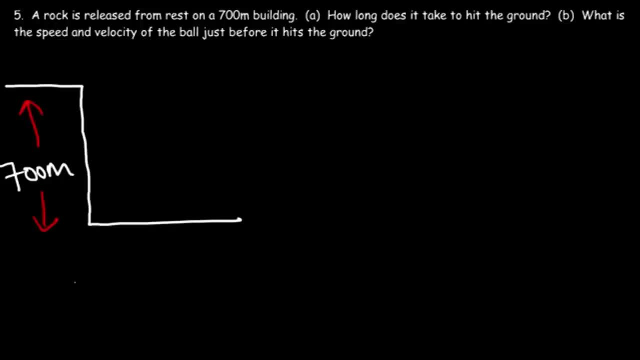 we got to find the time. let's make a list of what we have. the rock is released from rest, so the initial speed is 0. we have the acceleration in the y-direction, that's negative 9.8. we're looking for the time, but we do have the displacement, the displacement. 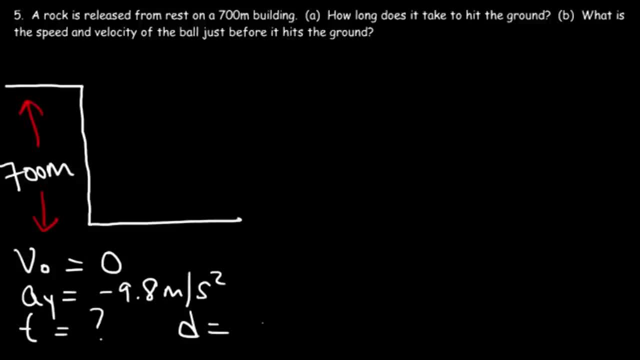 in the y-direction is not positive 700, but it's a negative 700 because the ball is moving in the negative y-direction. so let's use this equation: d is equal to the initial t plus 1, half a t squared. now d is negative 700, the initial fortunately 0. so 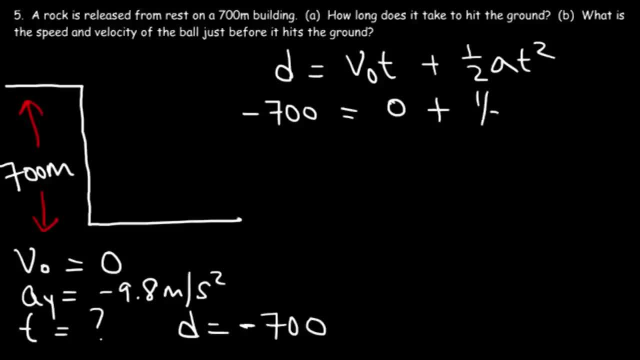 we can avoid using the quadratic equation. the acceleration is negative 9.8, so now all we got to do is find T. so half of 9.8 is 4.9. now to isolate t squared, let's divide both sides by negative 4.9. so 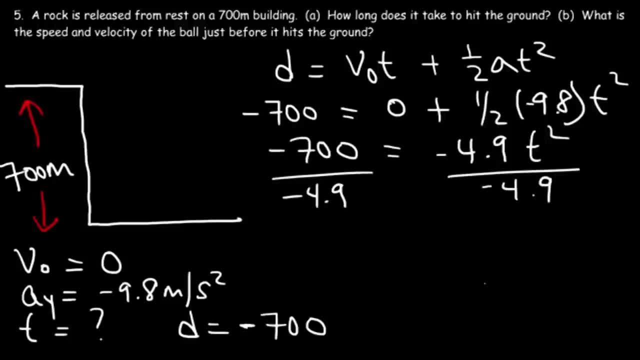 negative 700 divided by negative 4.9 is 142 point eighty six, and it's positive. so now let's take the square root of both sides. so T- I'm gonna write it right here- is 11.95 seconds. so that's how long it takes for the rock to. 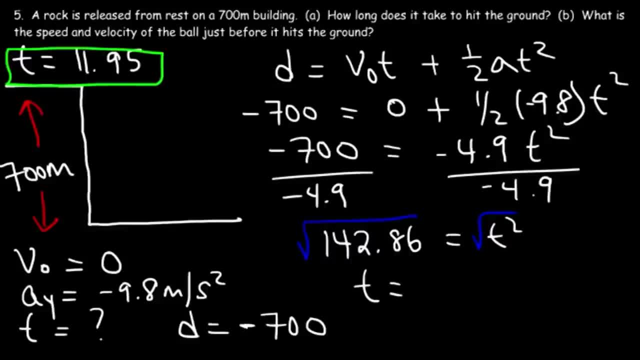 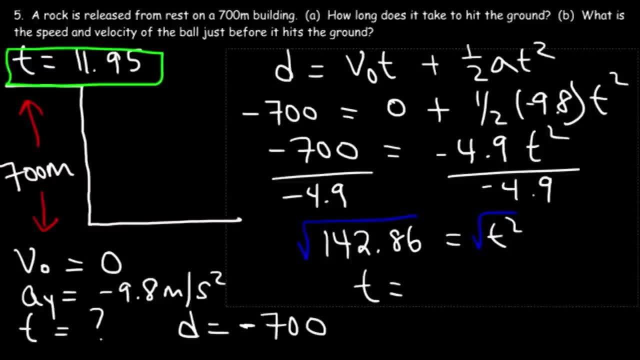 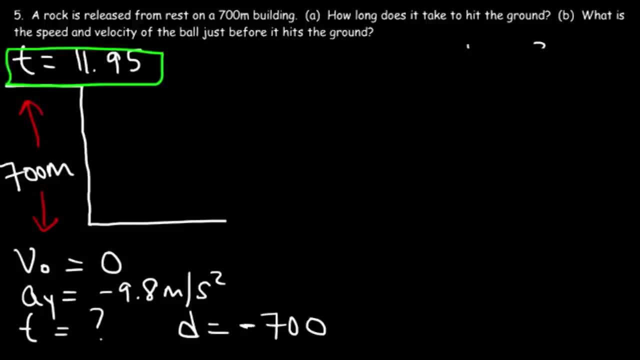 Part B is 11.95 seconds. how can we find the speed and velocity of the ball just before hits the ground? so we're looking for VF. in this case, we have the initial speed, we have the acceleration and we have the time. so therefore we can use this familiar.